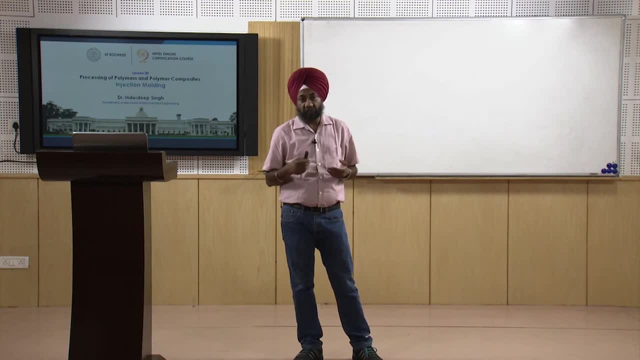 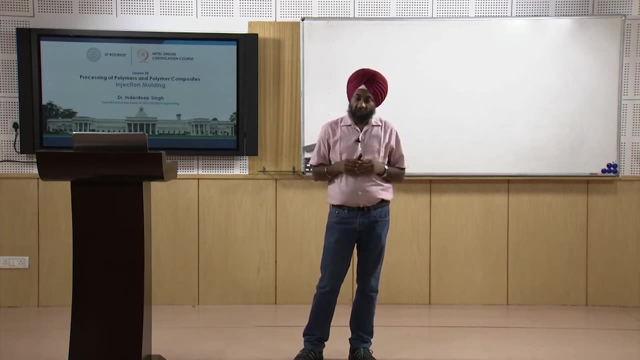 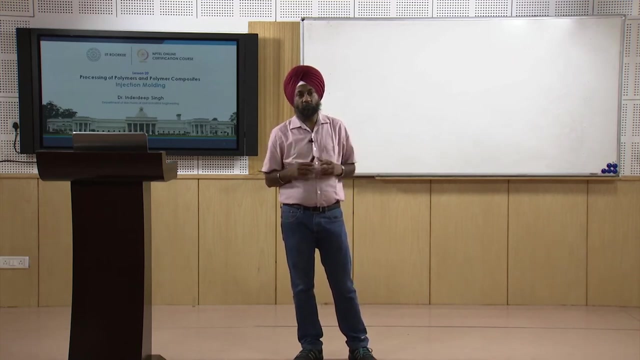 is the classification of composite materials? what are the challenges? in context of composite materials, We have also seen processes that are used for making the composite products And, if you remember, the very first process that we have seen was a hand lay up process And in hand lay up process we have seen it is a manual process. it is a widely used process. 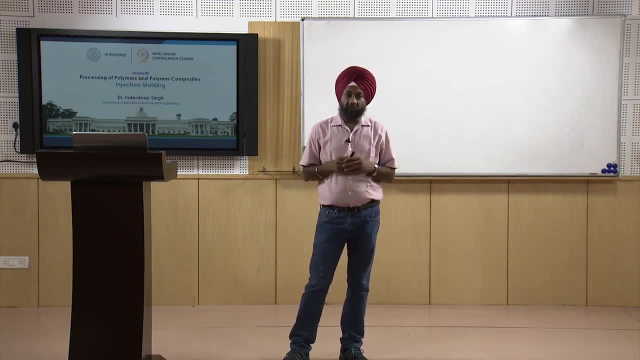 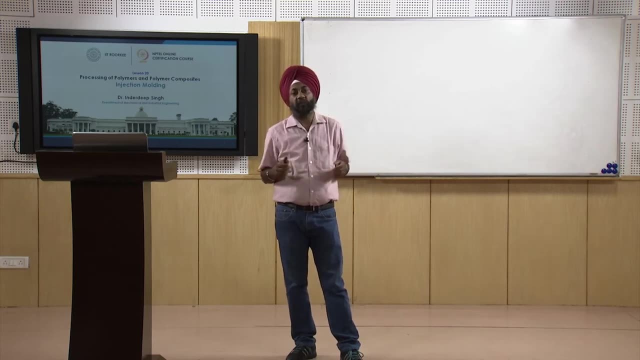 The shape of the product is slightly limited. we can make simpler shapes in hand lay up process, but the size of the product is unlimited. we can go for a very large size products in hand lay up process. So we have seen the process of making the composite products. 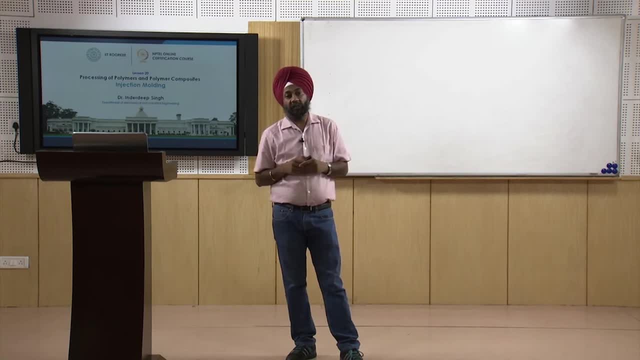 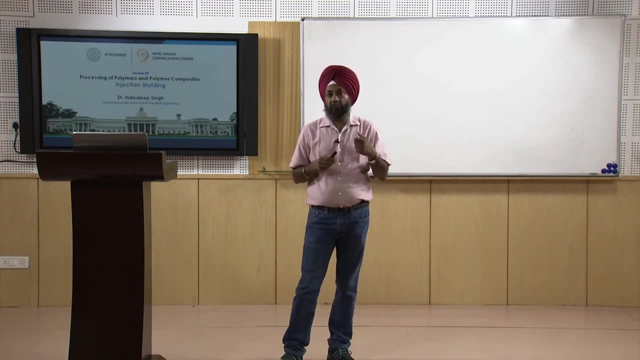 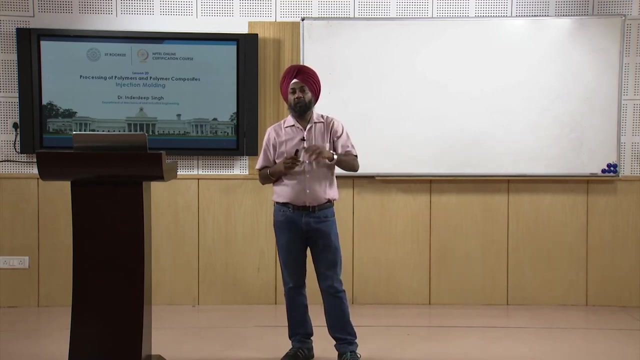 Then we have seen modification of the hand lay up process, that is, a spray lay up process In which short fibres are used. there is the chopper gun or a spray gun through which our polymer and fibre and the catalyst are mixed together and they are sprayed on the mould. So that is another modification of hand. 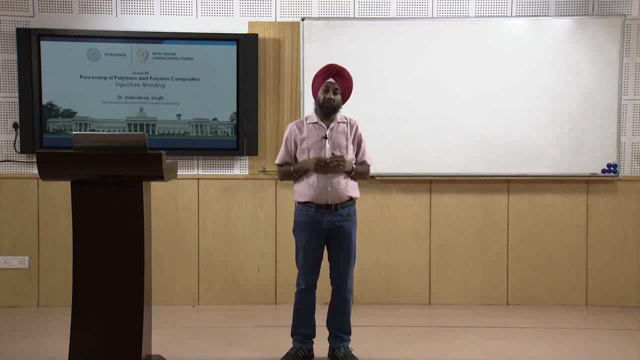 lay up process. Then we have seen, last in the last session, a compression moulding process, which is a commercial process, widely used process and is used for making number of composite products which are used in a aircraft industry, aerospace industry, as well as in our domestic applications. so we have seen three processes. so summarize. 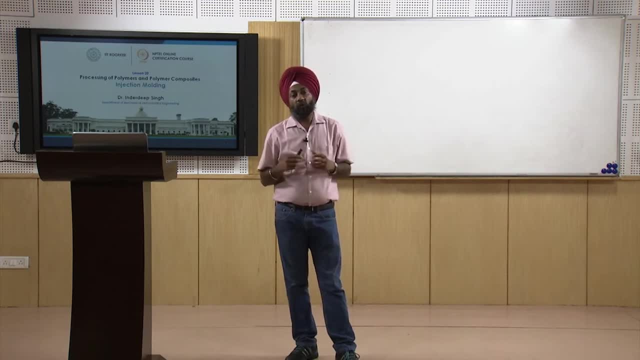 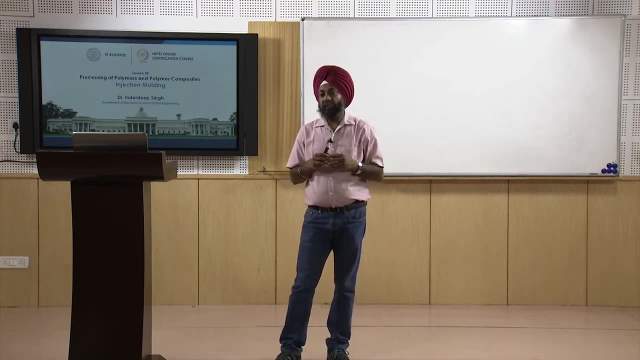 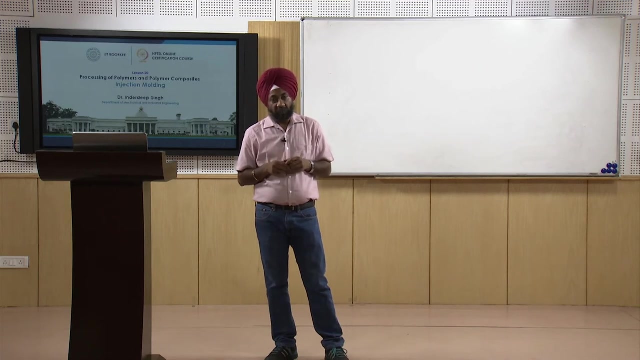 what we have covered. basically we have to see that how we can combine the fibers or the fibers and the polymers together. so basically the process has to have some mechanism through which the fibers and the polymers can be combined together in hand layer process we were using 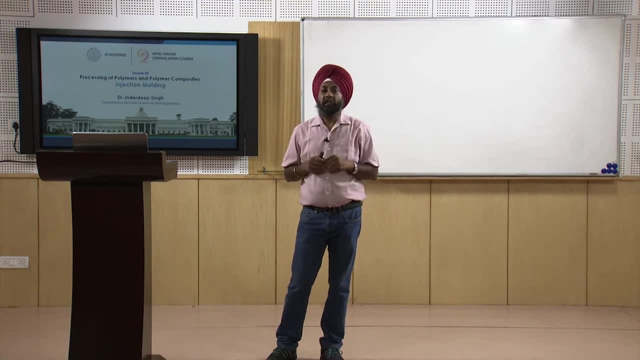 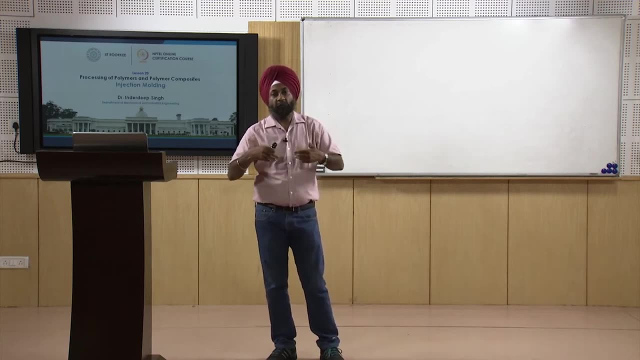 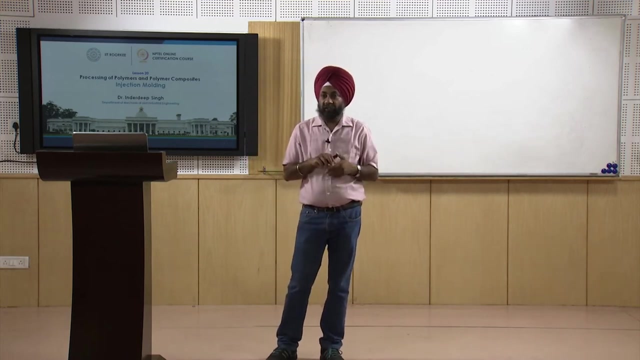 continuous fibers and we were laying up stacking of the mat of the fiber or the fiber mat, one above the other, and then we were applying the resin after each layer and then the four layers, six layers, eight layered layers were laid up in order to make a laminate and that 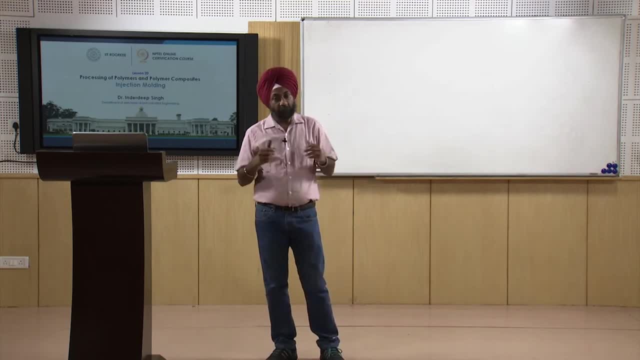 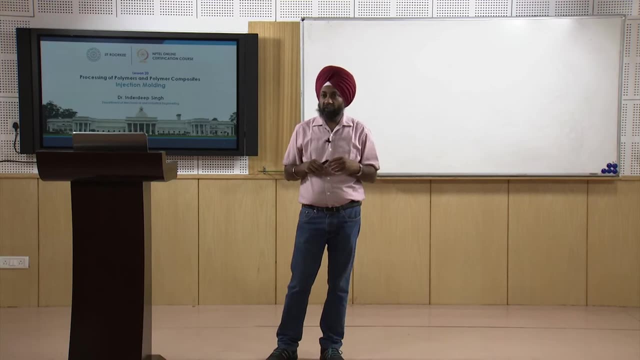 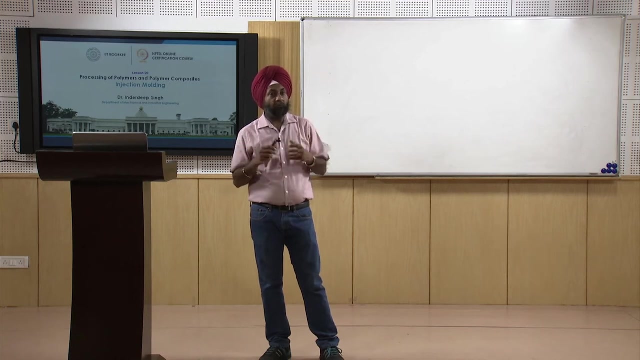 laminate was our final product. in compression molding also, we have seen both thermoset and thermoplastics can be molded and we can get a product which is a final product for any engineering application. so basically, we are combining the fibers and the polymers together to make composite products. 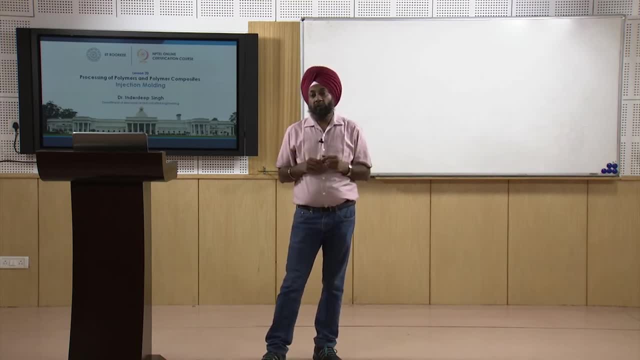 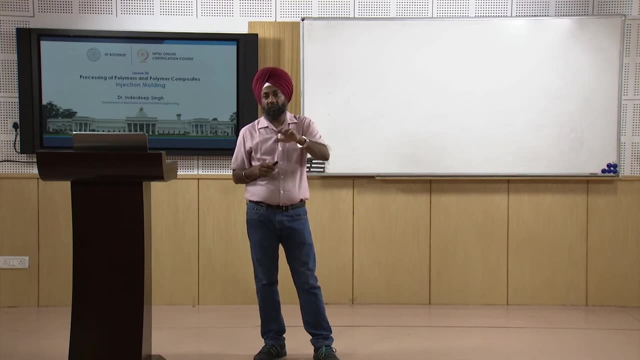 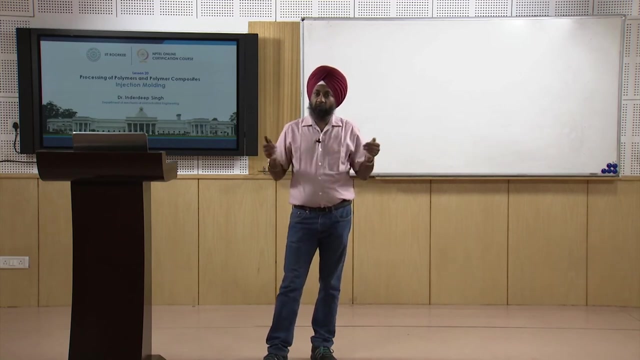 now from the classification point of view. if you remember, from polymers side we have two major classifications, that is, thermosetting polymers and thermoplastic polymers. from the fibers point of view there is a classification based on the long fibers: woven mat form, unidirectional long fibers. so from long fibers also there can 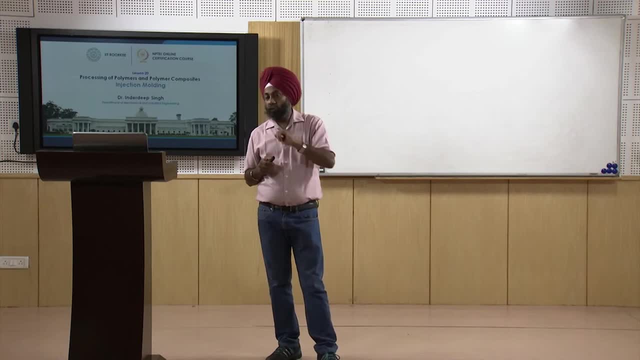 be two, three types of arrangements. then the opposite of long fibers is the short fibers, so we can have short fibers also, as in the example of spray layer process. you cut the fibers into small, small, small, small, smaller fibers in the chopper gun and these fibers, when impregnated with the polymer in the chopper gun, is deposited on the mold surface. 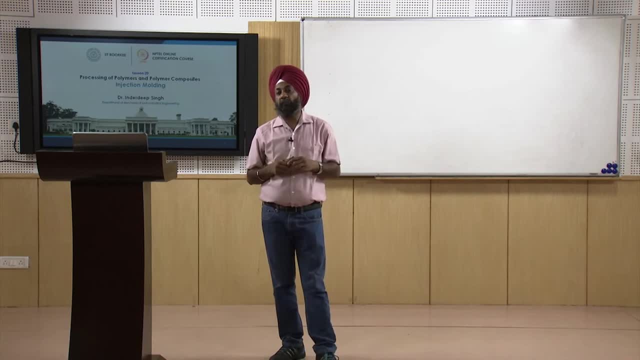 and we have seen a video also- a very good representation of polymers and thermosetting polymers and thermoplastics, also from the classification point of view. these are the ones which are used for short fiber reinforced polymer composites. so what is the analysis of polymers and thermosetting polymers? in the chopper gun one can see that the polymers 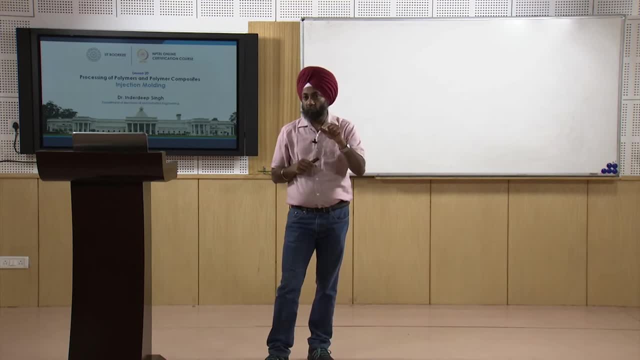 are used for short. several different purposes. only one is used for short fiber. very closely, of course, we can see that the polymers are used for short fiber: reinforced polymer composites. a lot of the polymers are used because they consist of very long fibers. they are used 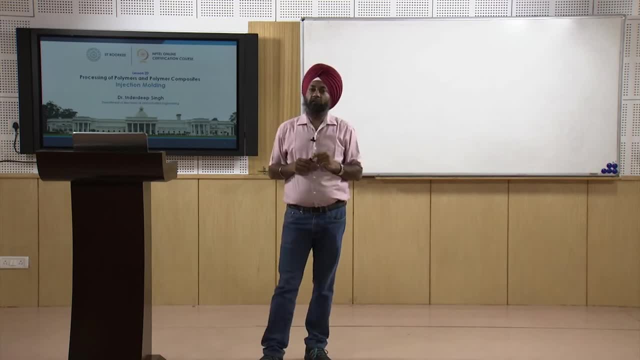 just for short fiber only, because they are existed long time. so that is what it is used for. it will take your time showing you cultural of them: small fibers for making the reinforcement and the polymer will be the thermo plastic polymer and, if you remember, we have already discussed the basic concept of injection molding. 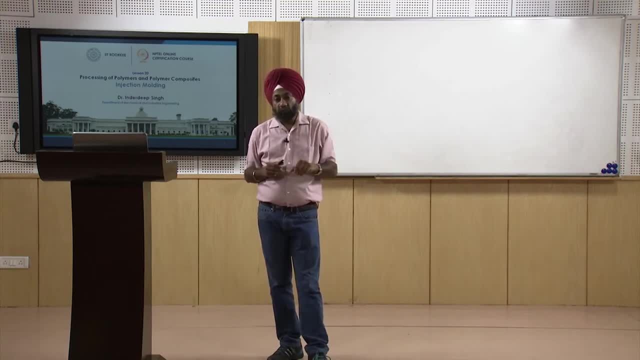 in our discussion on processing of polymers. so the basic machine remains same, the process almost remains same. only difference that we have to introduce here is that how to combine the pallets and the fibers together. otherwise the process remains same. the process details remains same, the process equipment remains same. only thing is the means and mechanisms. 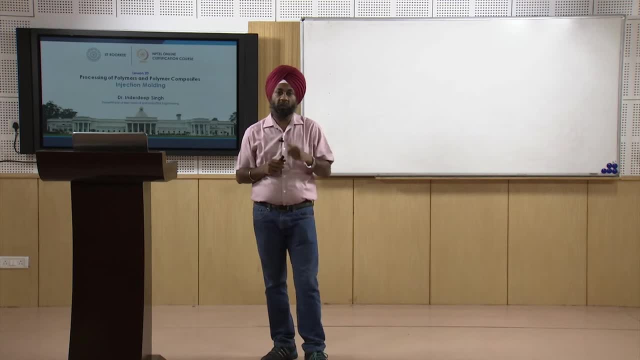 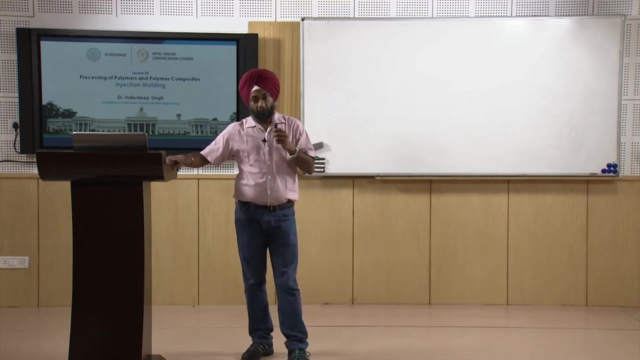 through which we are going to introduce the fibers into the polymer and, finally, what are the intricacies that are involved in this mechanism and what will be the type of the product that we will get in the injection molding process. so, basically, we have to focus our attention on the last point that i have highlighted, that is, how the fibers and the 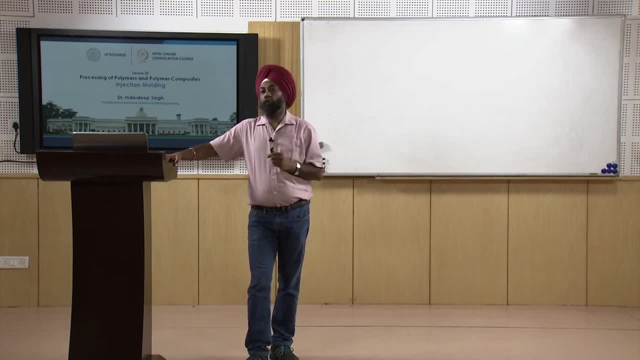 polymers will be mixed together. this is also a closed mold process. must i say that closed mold two processes we have seen: hand layup and spray layup. both are open mold processes. last session we discussed compression molding process, which is the closed mold process. now, currently we will be seeing today injection molding, which is also a closed mold process. 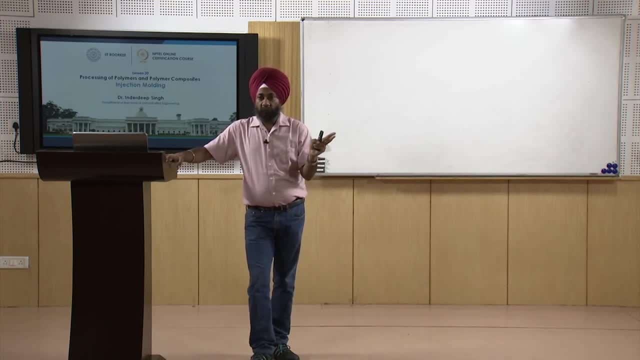 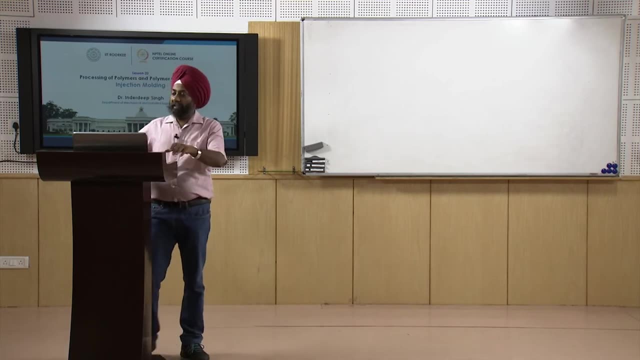 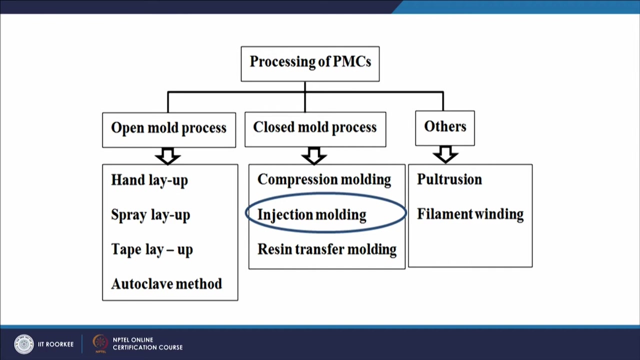 so till today we will have discussed two open mold processes and two closed mold processes. now let us first go through the discussion and the ppt. this slide is common to all our presentations on polymer composites. you can see the open mold processes two we have already covered hand layup and spray. 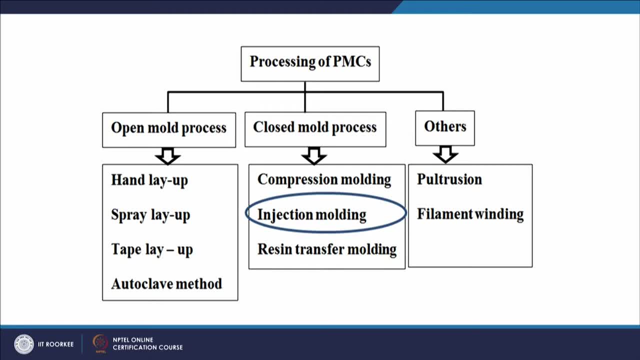 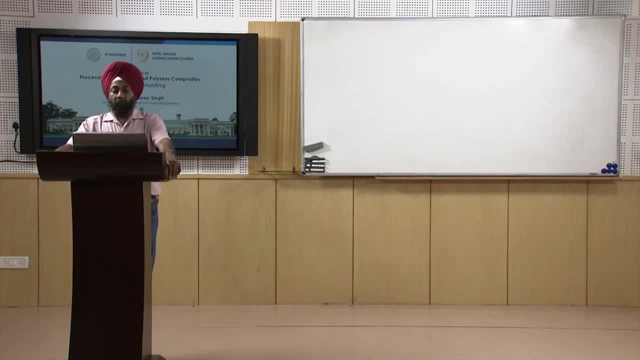 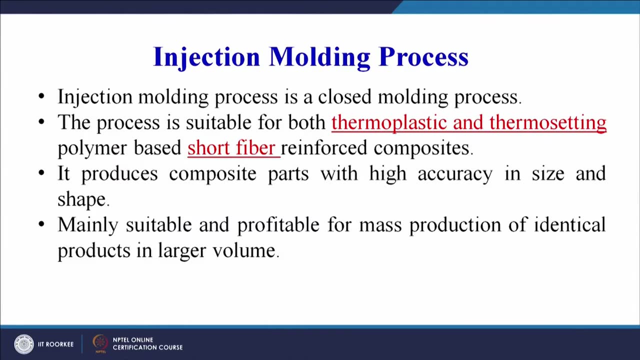 layup and injection molding is going to be covered today and the last session. we have covered the compression molding process, now injection molding. let us try to understand. it is step by step. injection molding process is a closed molding process. already the process is suitable for both thermoplastic and thermosetting. 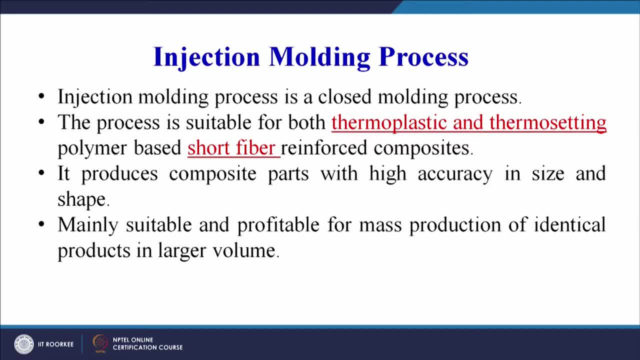 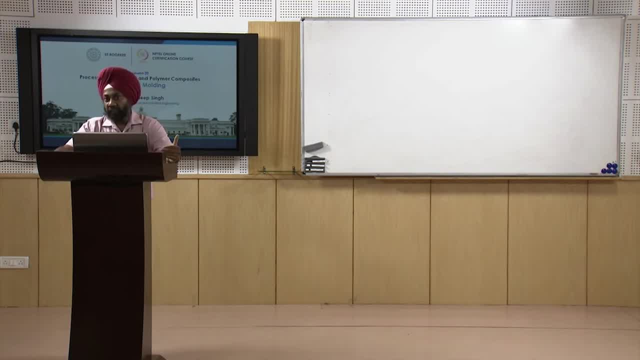 polymers, polymer based short fiber, reinforced composites. so majorly maximum applications are there for thermoplastic based composites but maybe under special circumstances we may also go for thermosetting based polymers also. but most of the applications. we will see that the process. 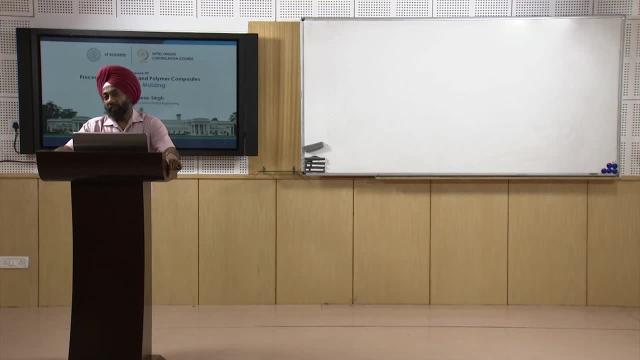 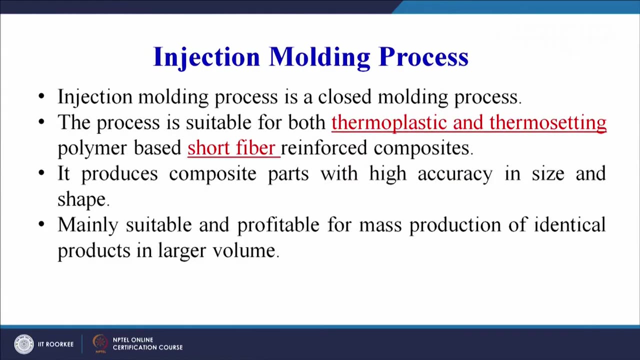 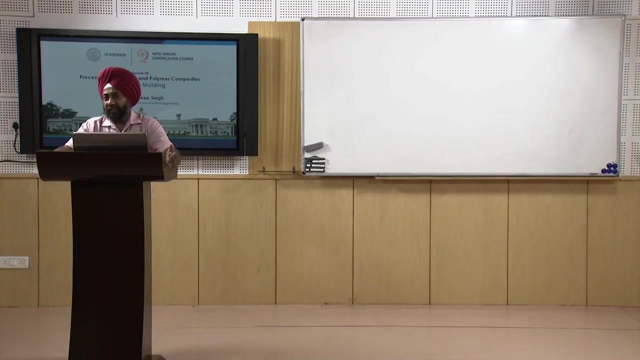 or the injection molding is used for making thermoplastic based short fiber reinforced composites. it produces composite parts with high accuracy and shape. so this is one thumb rule: wherever we will have a closed mold process, there will be a- you can say- characteristic advantage that we will get very good surface finish and very high dimensional accuracy. 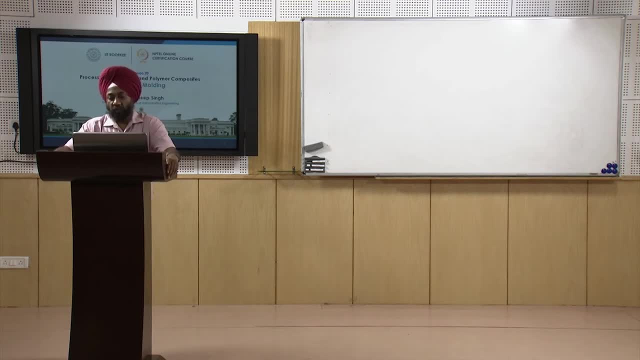 mainly suitable and profitable for mass production of identical products in large volume. so there are three things here: mass production, identical products, larger volume. larger volume is not in terms of the volume literally, but it is in the term of numbers of products that we are going to make. that is, mass production of the large number of parts. now the parts. 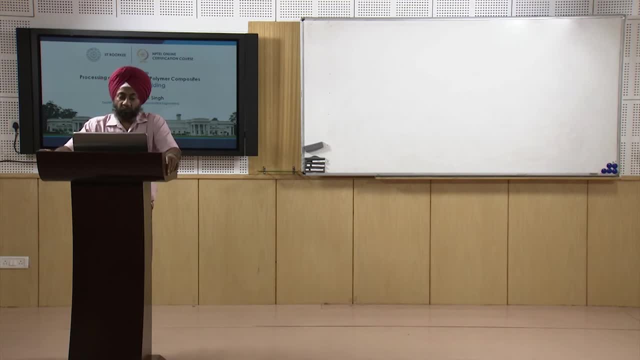 have to be identical. now, what is the bottom line in this particular point is that last time also, we discussed in our course on injection molding or in our session on injection molding that the die or the mold, is the most important part of any setup which is used for processing. 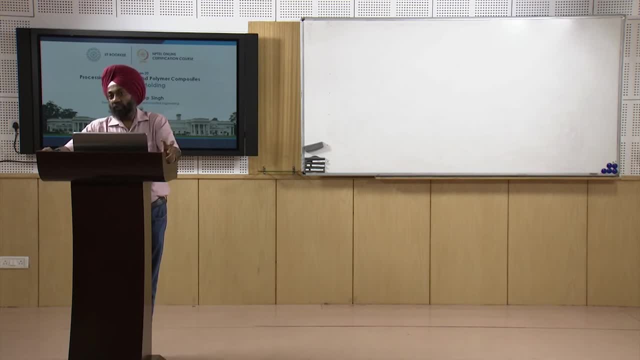 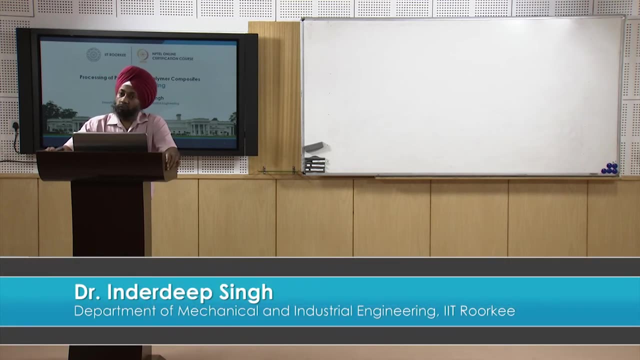 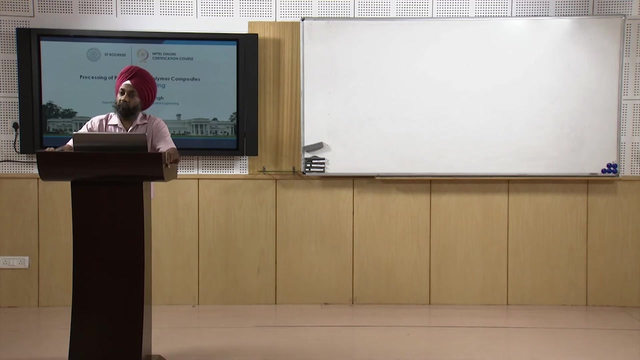 of polymers or polymer based composite. so the shape of the die, the complexity of the die, that is very, very important, and the cost involved is also most important. to consider any particular process now in injection molding as well as in compression molding, the cost of the die or the mold is very, very, very important. 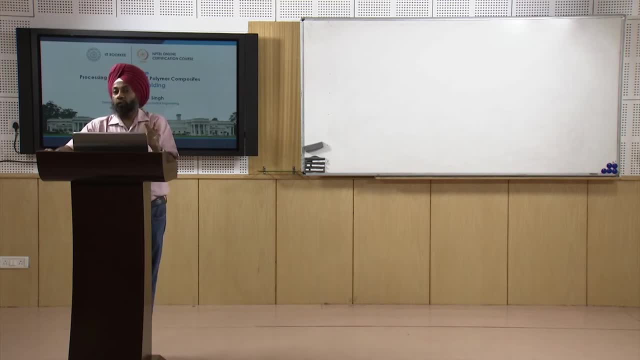 so the if, if we are going to make small number of parts, the cost of the die will not be justified. therefore, this process has to be used for large number of parts. only why? because the die is very, very costly and even the initial investment required to procure or purchase. 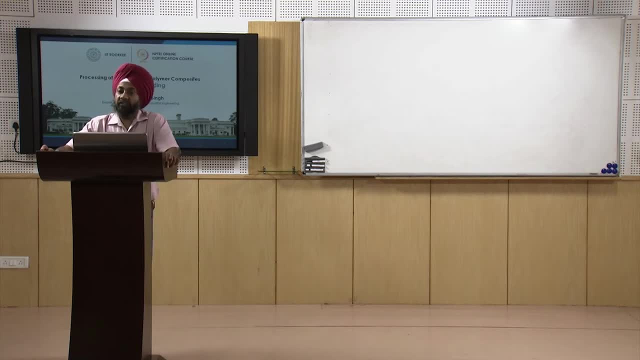 a injection molding machine is relatively higher as compared to the hand layup or the spray layup process. so, wherever we are going to make, another point that is going to come up in the subsequent slide is that this process is not used for very large size parts. so the point is that if the size of the product is not that large, 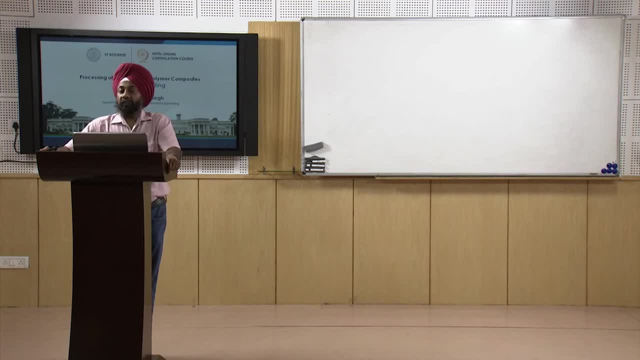 the number of products required is large. the complexity of the shape or the die is not that. ah, we can say. problematic means the shape is. we can control the shape, that is, the shape is not very, very complex, and then short fibers have to be used. we will easily think of only one process, that is, injection. 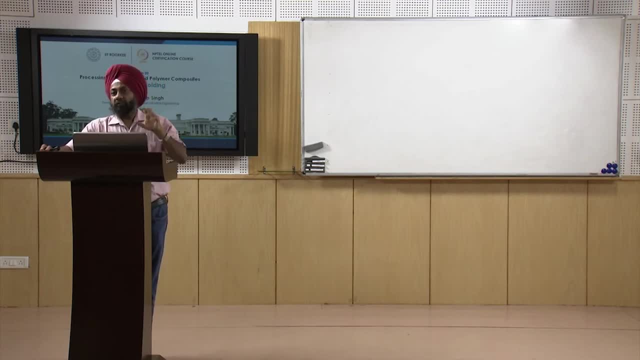 molding process. large number of parts size is not large, complexity of the product is not very high and the short fibers have to be used for reinforcement. i think in these four criteria we can very easily say that the exact process or the optimal process that should be used for such criteria is. 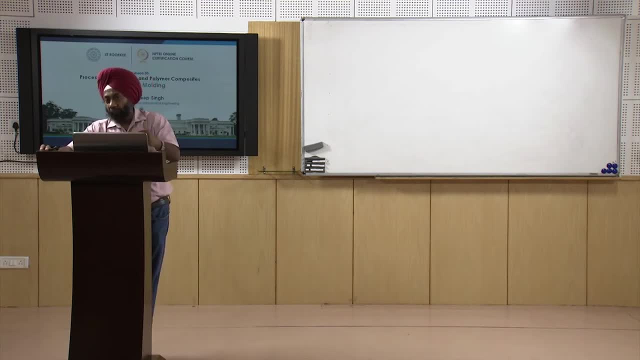 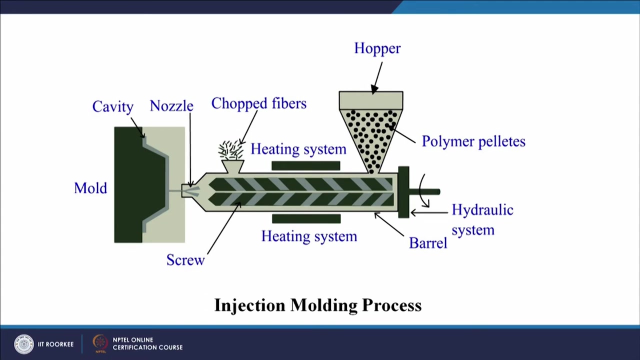 the injection molding process. so this is an point that we should always keep in mind- that the die or the mold cost, cost, cost is the very, very, ah, important criteria when deciding to procure a injection molding machine. on your screen you have a injection molding machine, or a set of this is a schematic of a injection molding machine. so here we can see the first. 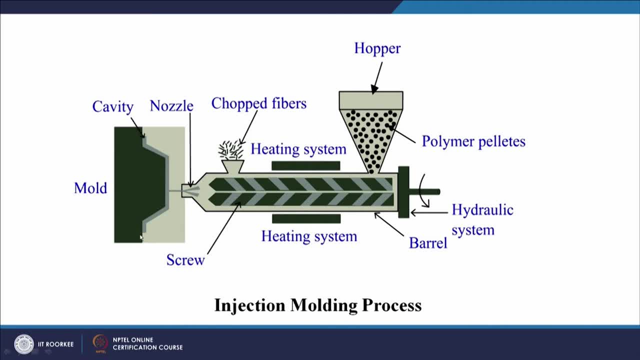 let us see the most costly part of this part, that is, the mould. the mould is in two halves. this light grey colour is one half of the mould. dark grey colour is the other half of the mould, and when the two halves of the mould close in between, we get a cavity. exact replica of the final product that we 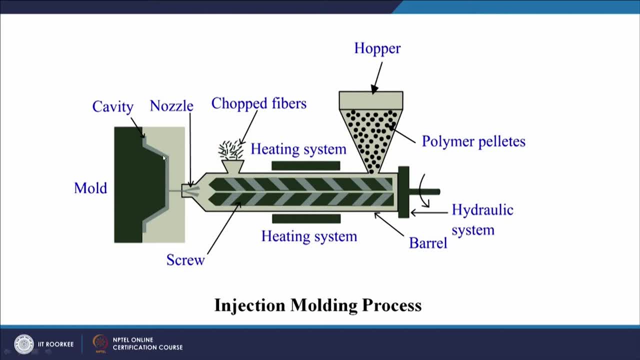 want to make. so, in between, this is a cavity. this is a product that we want to make now. here you can see. the other system more or less is same, only addition is the chopped fibres. this is the chopped fibres that you see on your screen now, as per the process, 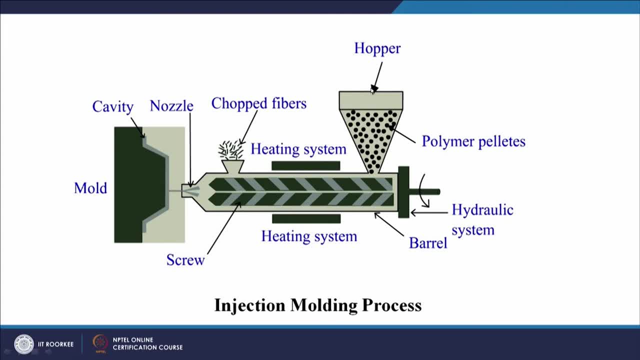 details. as we have already discussed, we will put our polymer palettes. the black colour polymer palettes are shown here. so these polymer palettes we will put in the hopper and through hopper they will be coming into the barrel. now there is a heating system, all. 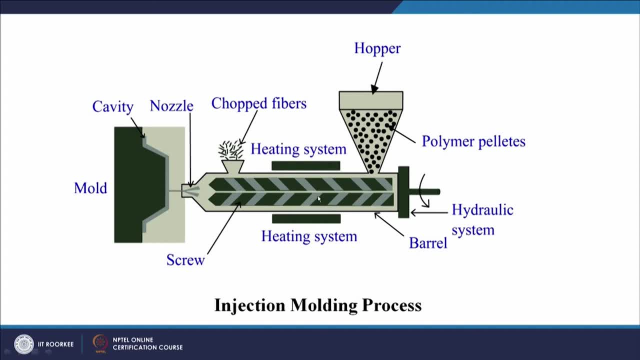 around the barrel which will heat these polymer palettes and they will be converted, or they, the polymer palettes, will melt and they will be moved forward by the screw. and here we can see there can be a hydraulic system or there can be a screw system. so here a screw. 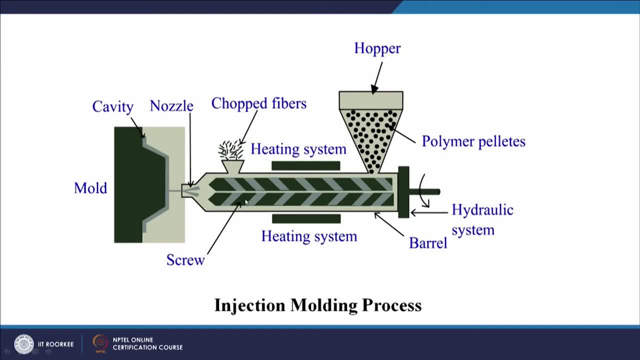 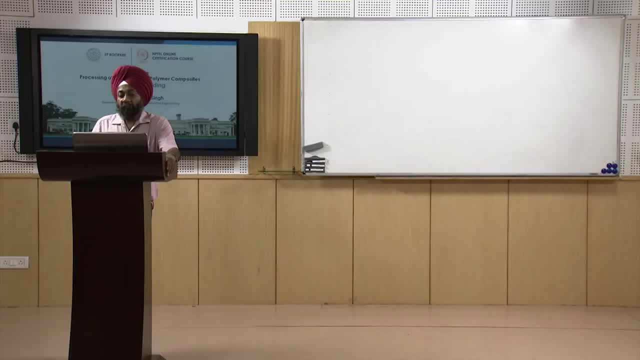 is shown here, the screw will rotate and it will push the polymer melt forward towards the mould or the die. as the polymer will move forward along the rotation of the screw, we are feeding the chopped fibres from here. these are the chopped fibres being fed from here. you can 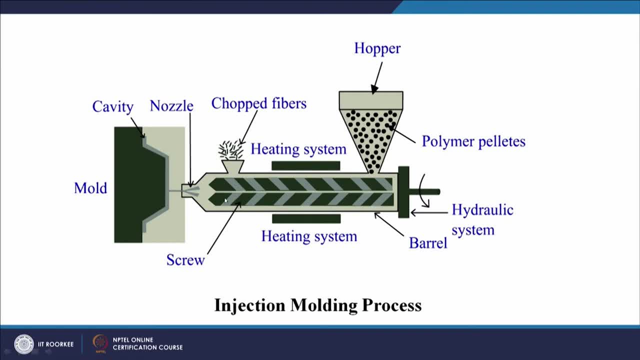 see, they are small size fibres and the fibres will mix with the polymer here and they will be pushed through the nozzle into the mould cavity. the mould cavity is generated between the two halves of the mould, as we have already seen. so this is the process of introducing 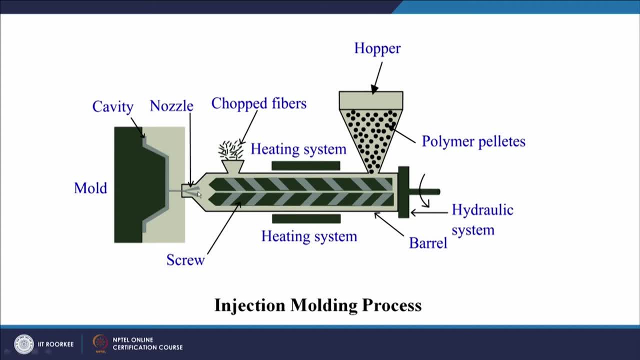 the fibres just before the polymer is going to enter into the mould cavity and we have to ensure that the fibres are uniformly distributed inside the polymer and we get a uniform composite product. so that is the basic process. now there can be other variants of this process, which 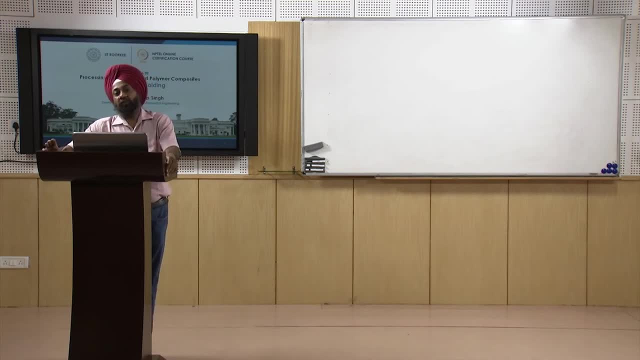 the, for which we do not have the diagrams here, but i would just like to briefly highlight what can be the other variants for extremely small size of fibre: 1. 0.. small size of fibres. we have these pellets that are already available and in these pellets 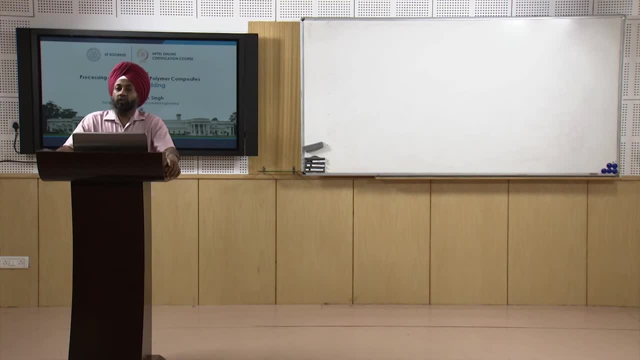 the short fibres are pre impregnated. so we have short fibres already in the pellet form and we get maybe pellets with glass fibres. for that we need not have this mechanism of introducing our fibres here. it will be a solid barrel without this mechanism. so the pellets 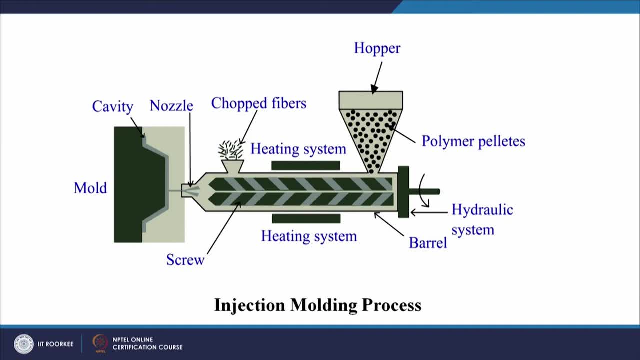 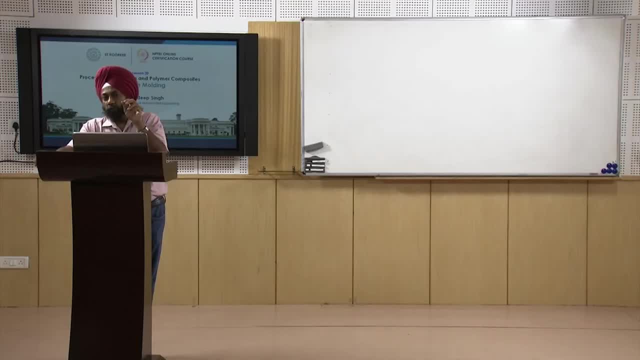 itself will have the fibres. so these are extremely small fibres which are there in the pellet form. so we will have a polymer also. we will have a. we will have a fibre also inside the polymer pellet and it will be introduced directly from the hopper. now, these pellets, 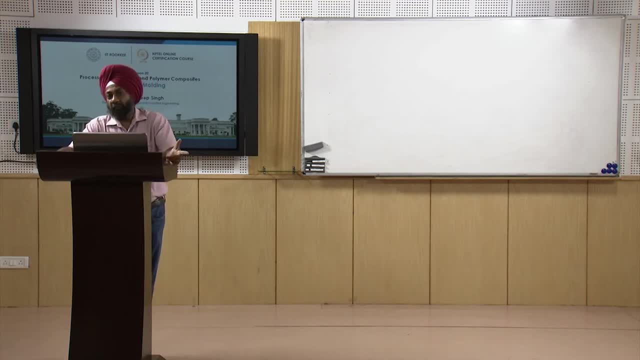 prefabricated pellets will have both fibres and polymer and when it will enter into the barrel, the polymer will melt because of the heating system and this mixture of fibres and polymers will melt, So it will move inside the barrel and it will be pushed into the mould cavity by the 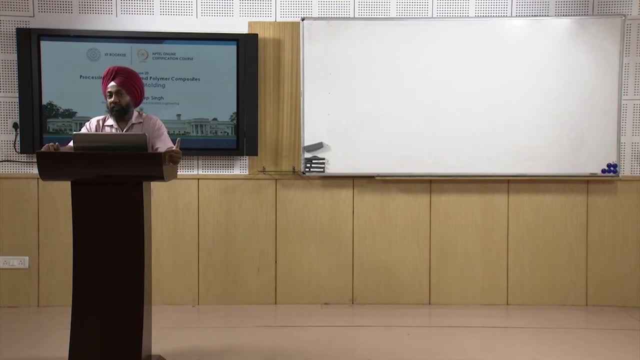 screw or a piston cylinder arrangement, so that kind of flexibility is also available, in which the fibre laden pellets are already available from the market. then there can be third mechanism or third variant of this process of introducing the short fibres into the polymers through the hopper only. 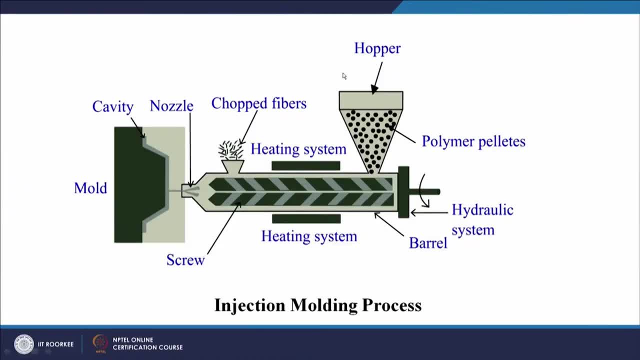 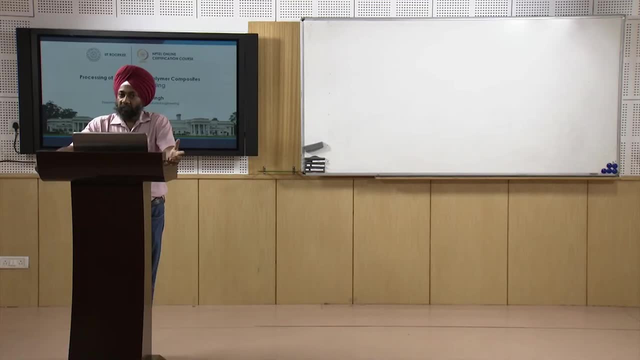 We can introduce our fibres. We can introduce our fibres directly in the hopper, but what can be the problem? you can just have a ah thinking in this direction, that if we put our fibres directly in the hopper, what can be the problem. you can just think over it. the problem basically will be: 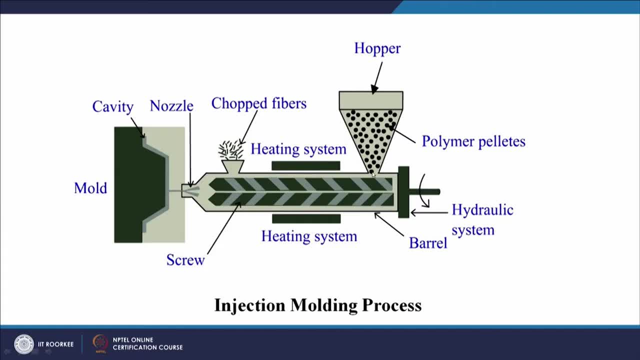 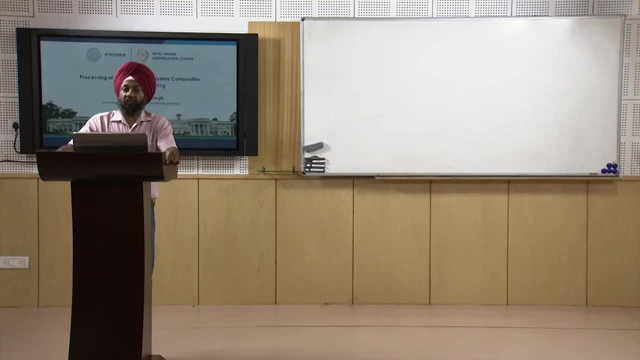 that the fibres that are introduced at this point, just below the hopper, will have to travel this much of distance, Because it is technically useful actually to remove those flying things that are's inserted in the hopper, in the hopper, so that they can be dragged down to the side instead. 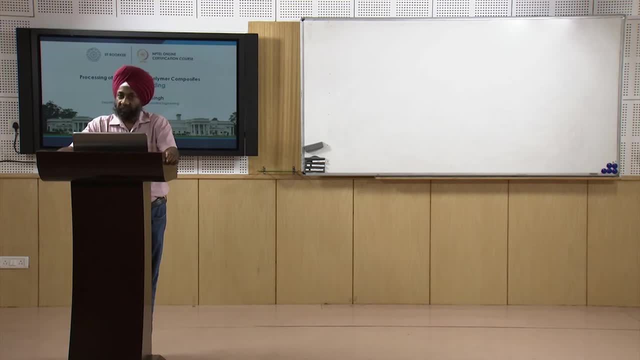 of there. So when the meat of a psyllium part has been crochets down, let us try to deliver other peculiar properties, such as in case, if you haveowi, can you turn the hot piece of philosophies to this side in this case, and so on. 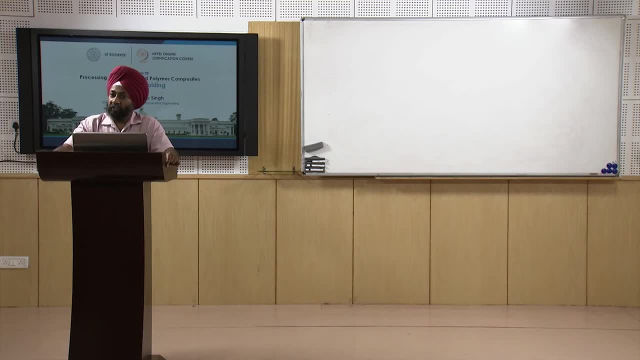 Now we can explain one kindof problem, of the problem we can get, which can be now, if e is actually possible to heat these fibres, shearing of the fibres may reduce their length and may cause damage to the fibres and the. 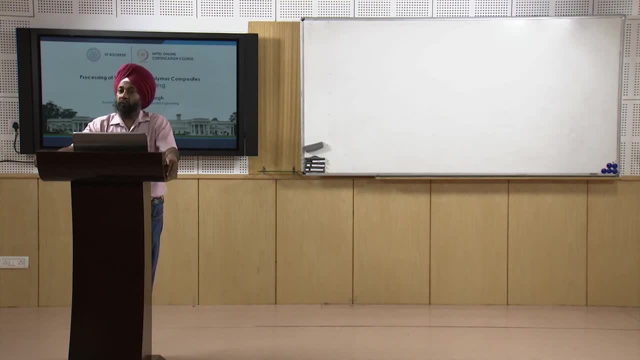 fibres may not be able to achieve the purpose for which they have been introduced into the polymer. So, basically, there are number of studies available in which the fibre is introduced along with the polymer pellets through the hopper, but it has been reported that there 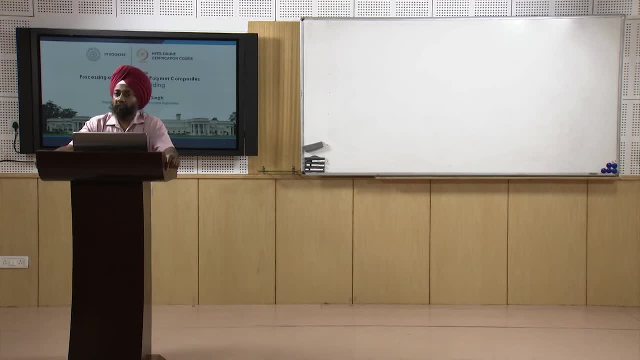 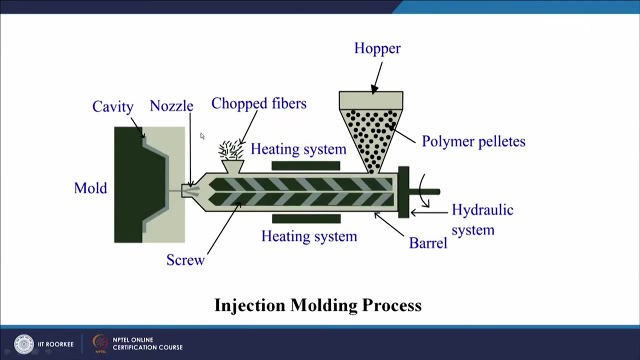 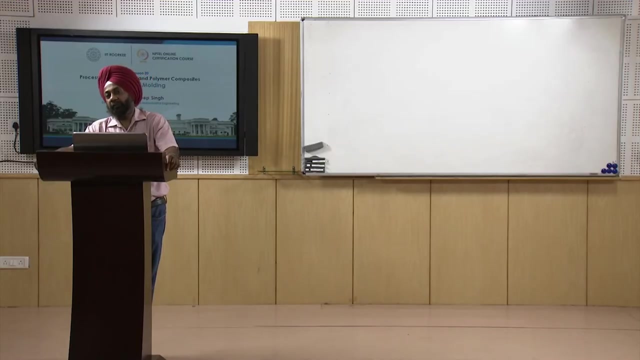 is certain amount of degradation in the properties of the fibre when they move through the barrel alongside the polymer. Therefore, the advanced version can be that you introduce your fibres just before the polymer is going to enter into the mould cavity, so that the fibres do not travel a long distance. 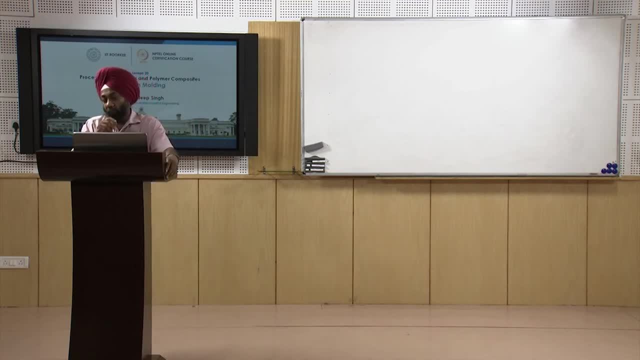 inside the heated barrel. So that is one may be process modification which is being used. So I think we have seen the latest modification in the injection moulding setup for introducing the fibres into the polymers. So this is the most important thing. 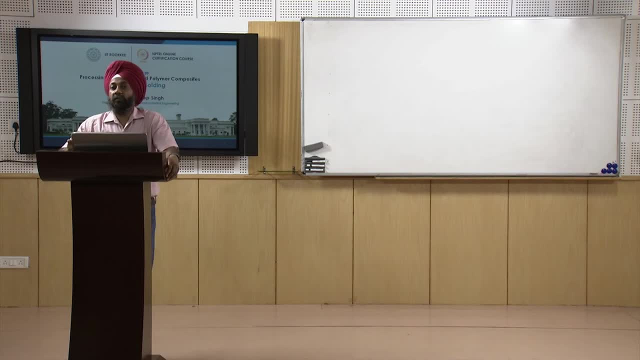 We need to understand regarding the introduction of the fibres into the polymer. otherwise, the standard injection moulding process is well known. I think most of you may be knowing. for those of you who were not knowing, at least in this course the learners have got an idea. 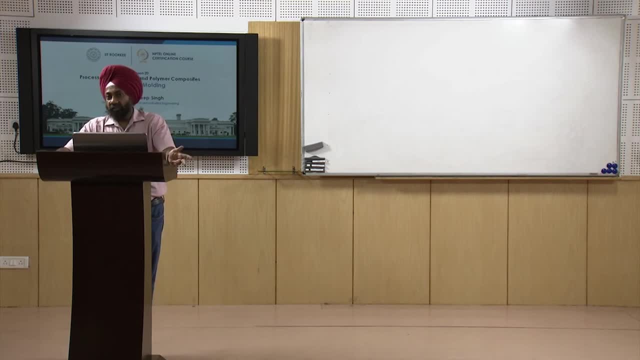 that what is injection moulding of polymers. in the last session in the ah may be in in our sessions on processing of polymers we have covered the injection moulding process in much more detail. So today I think I want to emphasize on this aspect only, that how the polymer will be ah reinforced with. 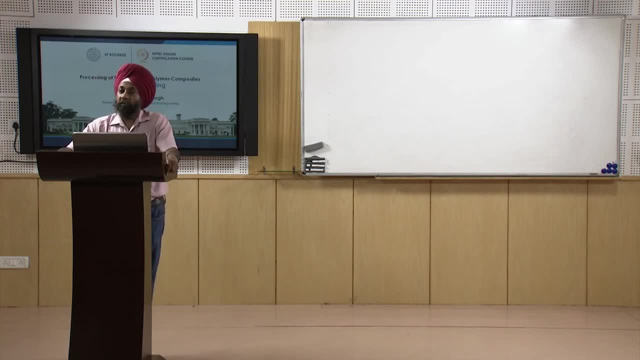 the natural fibres or the synthetic fibres, and how the fibres will be introduced into the polymer, and I think I have tried to explain this with two or three variants of the process. Now, coming on to the procedure I have already explained, So we will have a ah glimpse of certain finer points in the form of sentences, so that we 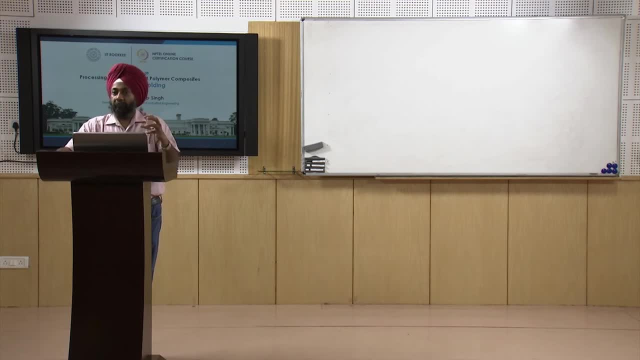 understand- We keep this in our mind, we remember this for a long, long, long, long period of time- that how the fibres are introduced into the polymer. So the fibres and polymers are either pre blended or mixed manually and fed into the hopper. 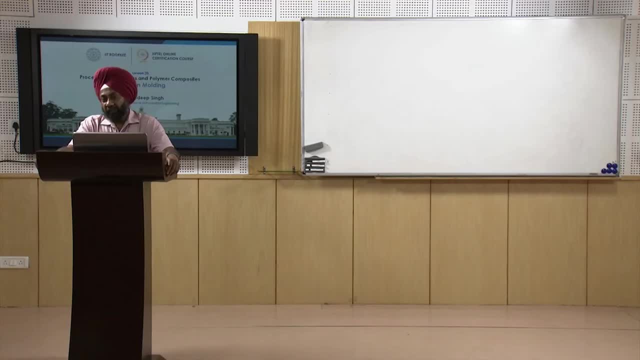 Now two points are important here. pre blended- yes, there are pellets which are available. or pre blended pellets are available which have the fibres- very small size fibres- pre blended into the polymer, So directly. then the process becomes very simple. we have to buy these pellets and directly. 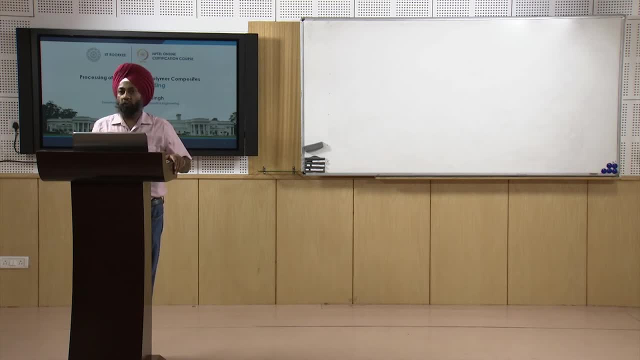 put these pellets into the hopper and then our process will automatically we ah running and the fibres and polymers will move through the barrel into the mould cavity and we will get our product. or the second point is we can mix the fibres and the polymers in the 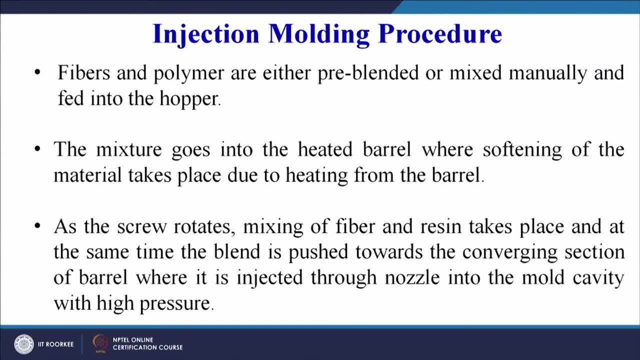 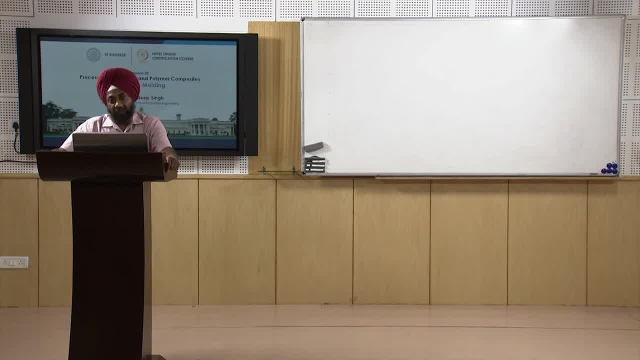 hopper and then the fibre and polymer will come from the hopper into the barrel and then they will be pushed forward, pushed forward the because of the heat. the polymer will melt and it will be pushed forward into the mold cavity. so that is another thing. so two variants. third variant, as we have already, 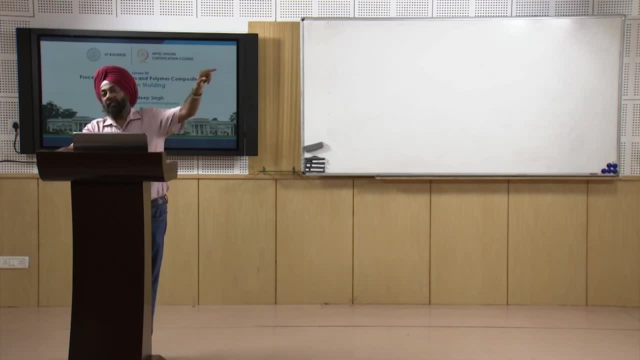 seen the diagram that the fibers are introduced separately just at the end of the barrel, just before the entry of the polymer into the mold cavity. so that is another variant. but there are the limitation. i think it might have occurred to your minds also that what can be the limitation? 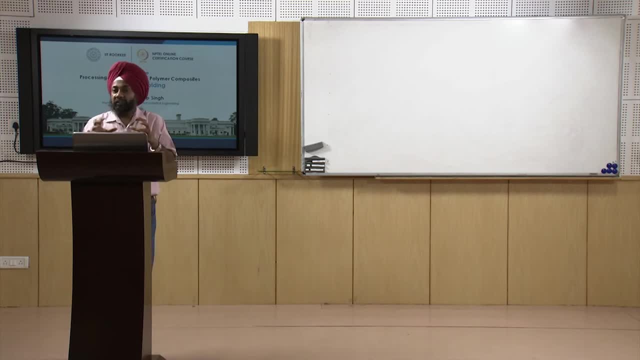 there the blending of the fiber and the polymer is is getting very less time because we are just introducing the fibers before the entry of the polymer into the mold. so the fiber and polymer is getting very less time for having a handshake or for having a friendship or for developing a friendship. so that time period may be one of the limitations in that. 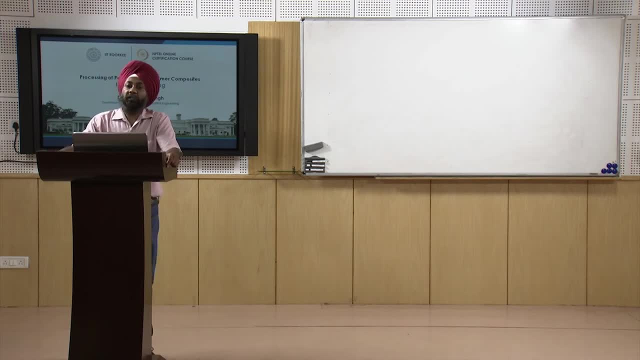 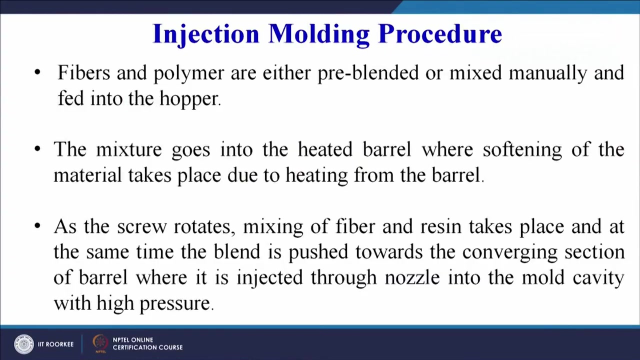 case when we are just introducing the fibers before the entry of the polymer into the mold cavity. so that can be one limitation there. but yes, different methods have been used and have been found successful for different combinations of polymers and fibers. so the mixture goes into the heated barrel where 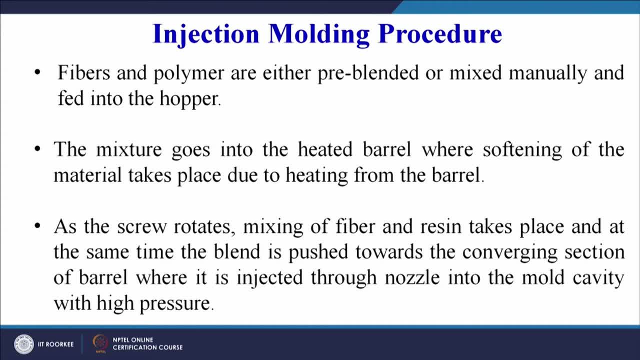 softening of the material takes place due to heating from the barrel. all of you know that as the screw rotates, mixing of fiber and resin takes place and at the same time, the blend is pushed towards the converging section of the polymer and the polymer is pushed towards the converging section of barrel, where it is injected through the nozzle into. 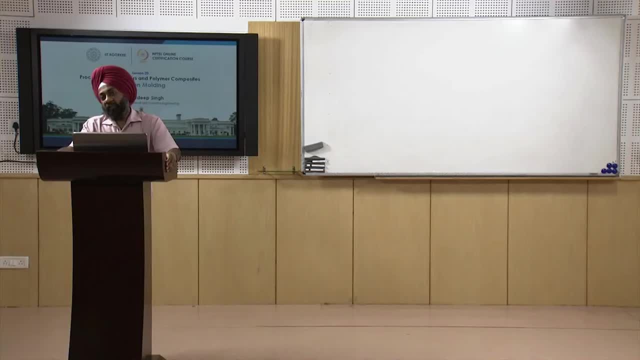 the mold cavity with high pressure. so i have already explained: from the hopper we get the raw material, it enters into the barrel, a screw arrangement rotates this mixture and because of the heating arrangement the polymer maybe is softened and then it is pushed forward and through the converging section at the nozzle the material is pushed into the pushed 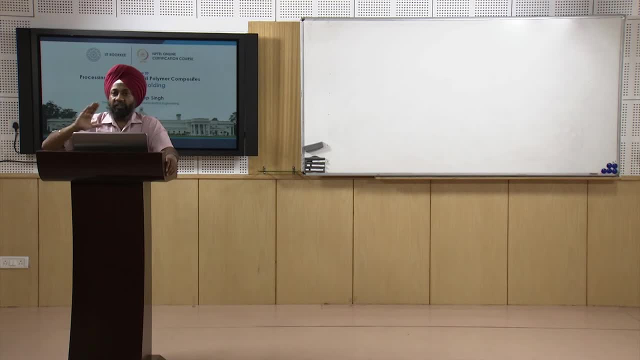 maybe or, as the name of the process suggests, Injected into the mold cavity at very high pressure. Now why high pressure is required? because the polymer has to go inside the mold and reach to the farthest corner of the mold. if you do not apply pressure, the polymer may 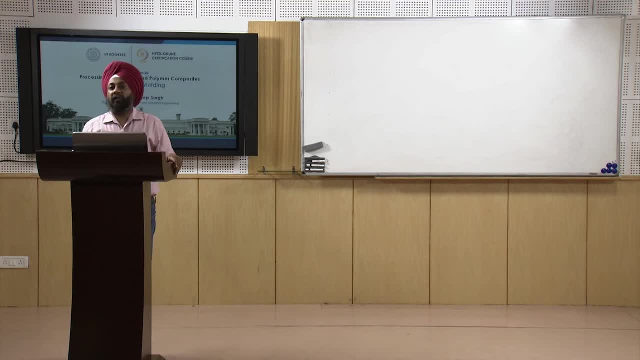 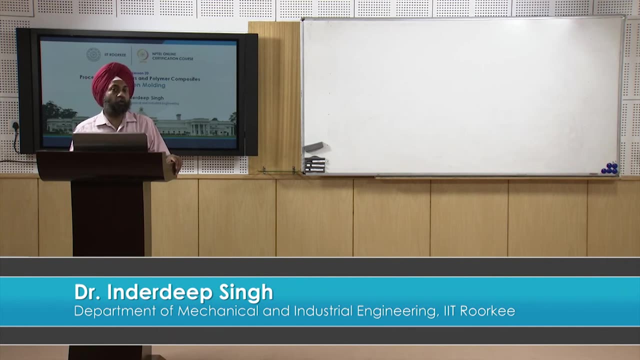 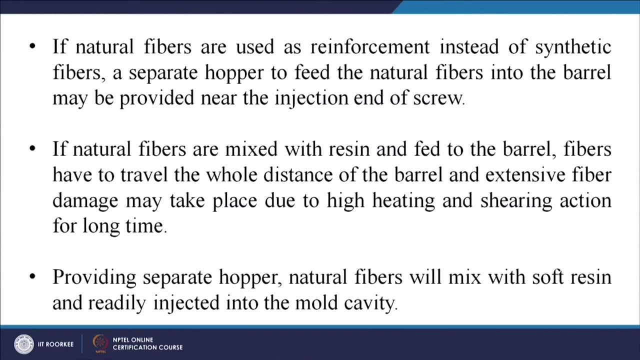 not have the velocity to enter into the farthest or the thinner sections of the mold and we may get a defective product. so we have to optimize the injection pressure also in order to get a good product. If natural fibres are used as reinforcement instead of synthetic fibres, a special case- 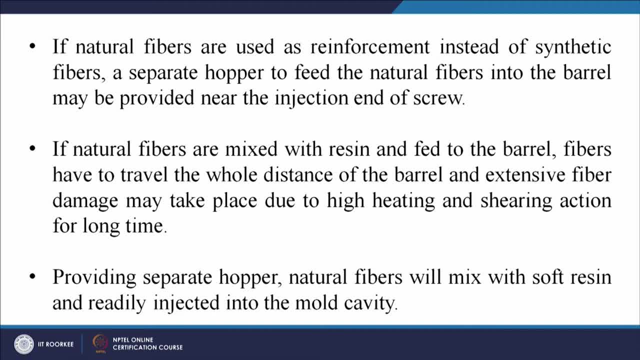 because we know that in case of composites we can have synthetic fibre reinforcement, we can have a natural fibre reinforcement. a separate hopper to feed the natural fibres into the barrel may be provided near the injection end of the screw, So that i have already explained that we may introduce the fibre just at the end of the 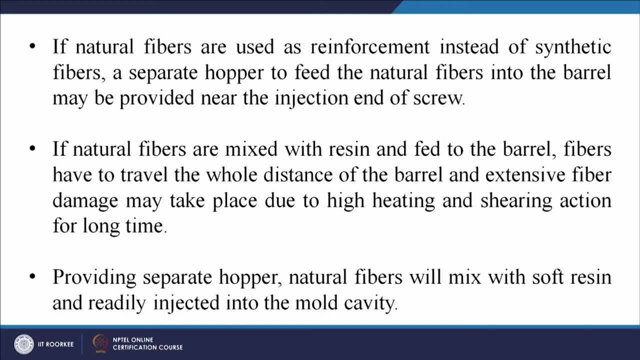 barrel So that the fibres and just mix with the polymer and enters into the mold through the nozzle. If natural fibres are mixed with resin and fed to the barrel, fibres have to travel the whole distance of the barrel and extensive fibre damage may take place due to high heating. 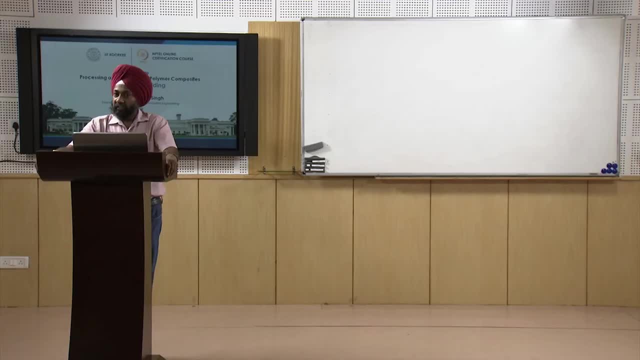 and shearing action for a long time. I have already explained that specifically for natural fibres, that is one of the limiting areas or one of the limiting issues. therefore, we try to introduce our natural fibre just at the end of the barrel, as was shown in our diagram, providing separate hopper: natural 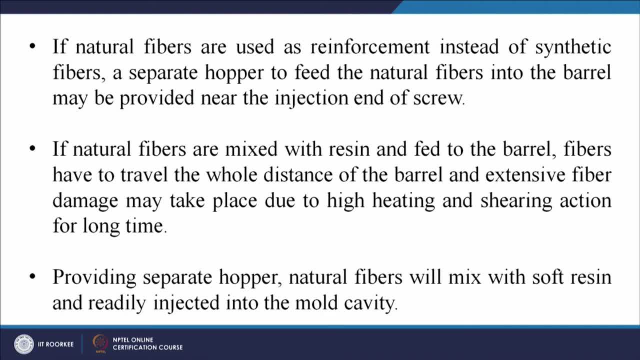 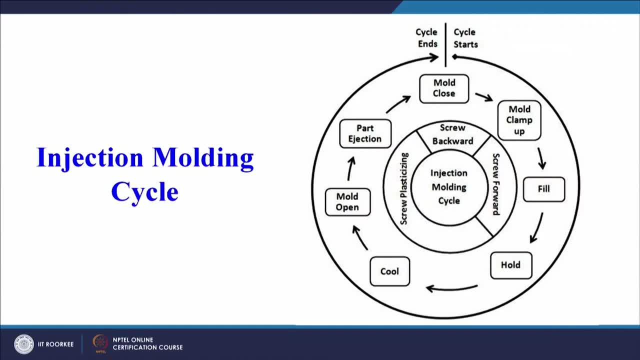 fibres will mix with soft resin and readily get injected into the mold cavity. Now this is a standard injection molding cycle, just introduced to revise the concept of injection molding. So on your screen you can see the cycle starts here, the mold closes. as soon as the mold closes. 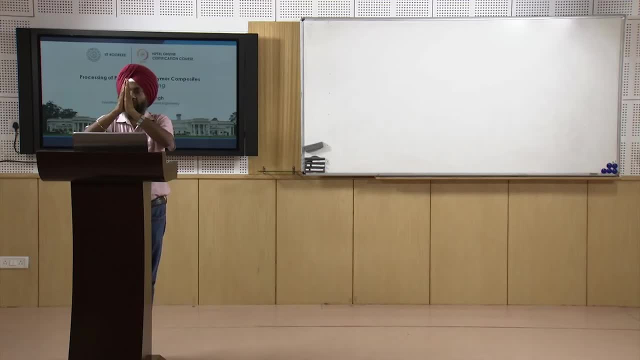 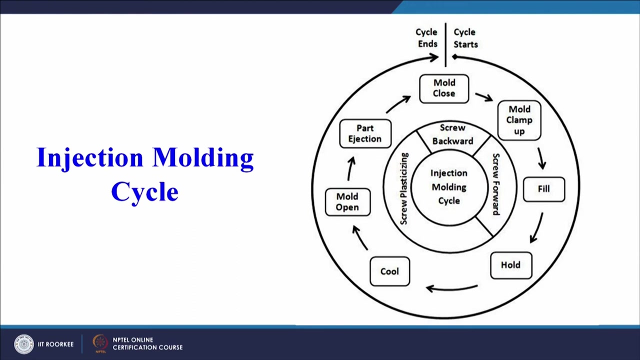 the cavity. The cavity is formed inside the mold, or the cavity which is the exact replica of our product is forms in formed inside the mold, So the mold closes. the cavity is now inside the mold. the mold clamp up So pressure is applied to keep the mold halves clamped. then we have to fill the mold with. 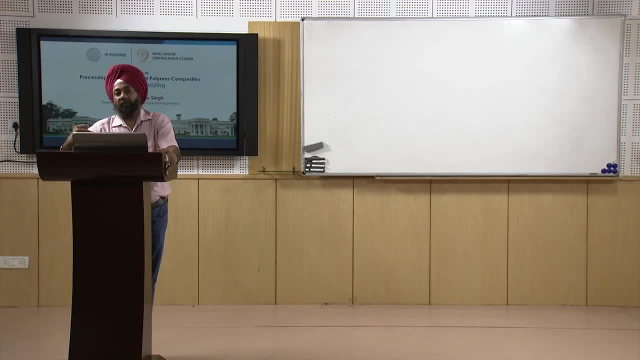 the raw material. now, raw material in case of our injection molding process is combination of a fibre and the polymer, So that is injected through the nozzle into the mold cavity. Then we have to keep the mold halves closed. that is called the hold or the holding time. 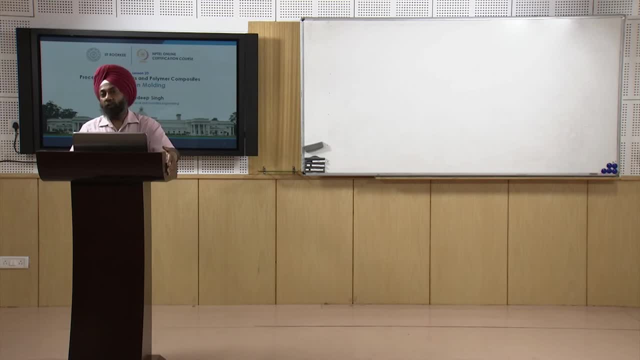 in order to get a solidified or a rigid or a stiff product. So we will give some time to the mold to remain closed so that the polymer filled with fibres inside the mold gets some time to solidify. keep the mold halves closed. it will lead to cooling of the material inside and solidification. 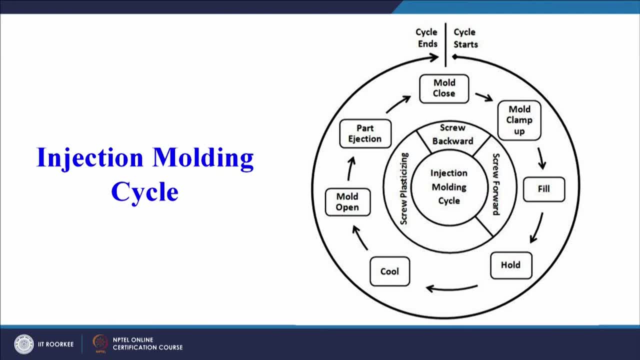 of the material. then, once the material has solidified, we will open the mold and the part ejection will take place. now, part ejection is sometimes facilitated with the help of ejector pins, as the polymer has the tendency to stick to the metallic mold. so if the material 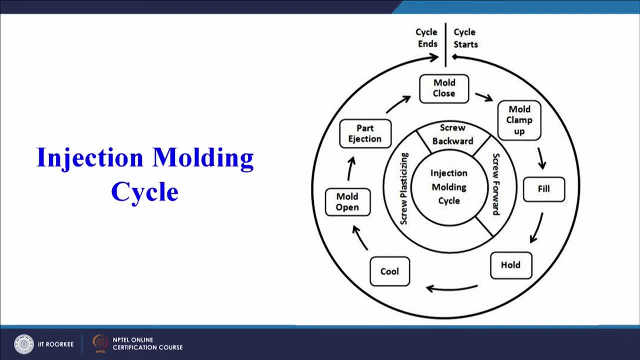 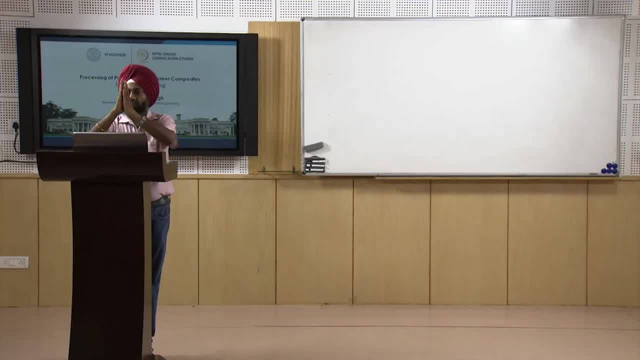 or the product may stick to the fixed half of the mold. so there are two halves of the mold. one is a movable half which will come and close the mold. other one is the fixed half. now the material may have, because of the shape, complexity, have a tendency to stick. 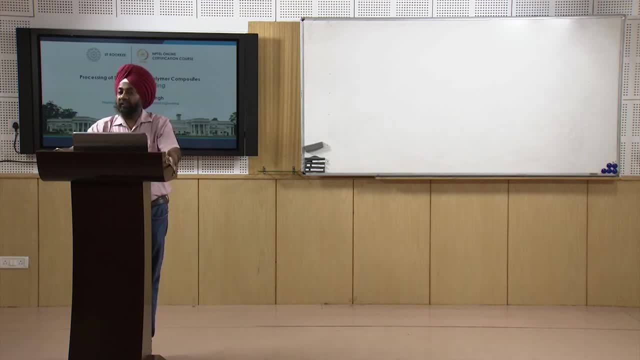 to one half of the mold. so wherever it has the tendency, we can have a ejector pins. ejector pins which will be hydraulically operated or pneumatically operated, which will just give a tap to the part, solidified, composite part or product and it will fall down into. 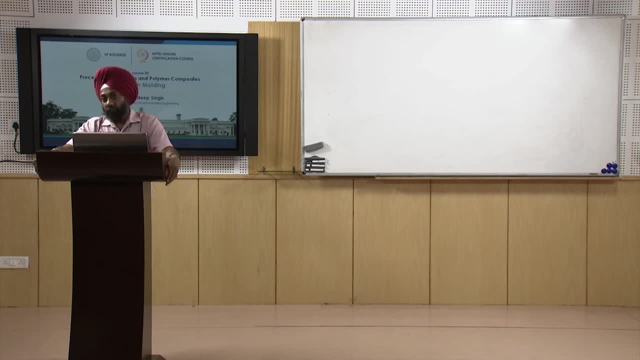 the collection bin or collecting bin. so that is one thing. that is part ejection. and once the part has ejected, the ejection will take place when the mold has opened up. so once the ejection has taken place, the mold is already opened. now the again the cycle will start. 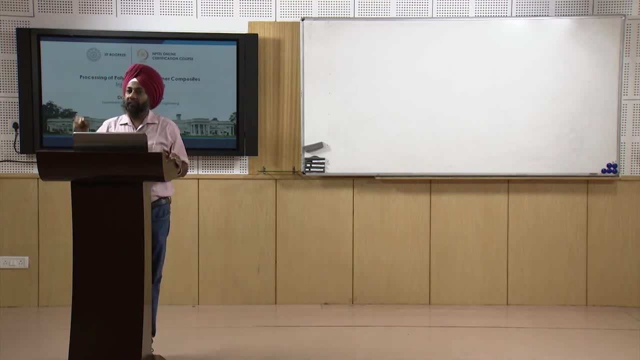 the mold will close again, we have the cavity inside the mold will be filled and the second cycle will start. so there are these three to four steps which are automatic in nature, and the process can be automated. before that we have to do some optimization. that at what? 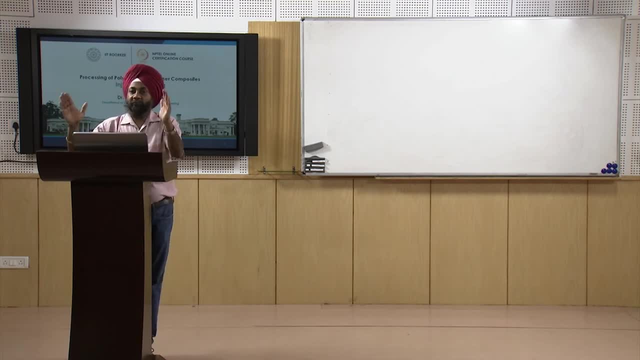 pressure we have to push the material? for what time we have to keep the mold closed? what is the back pressure? what should be the clamping force? so these are the operating variables that we have to keep in mind when we are designing the ejection molding process. 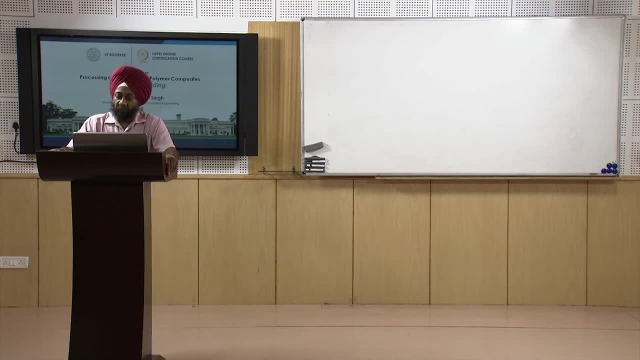 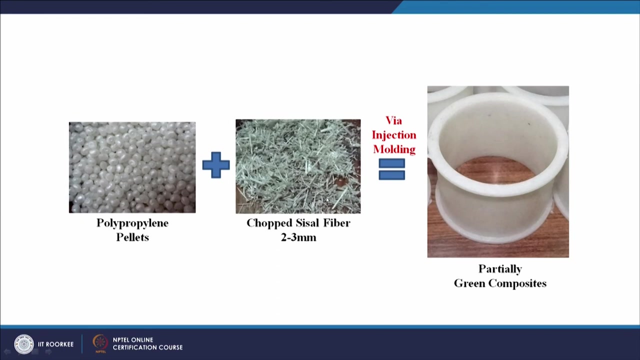 for a specific combination. So let us quickly see that how the composite products can be made. here we have a polypropylene pellets. this is a pellet form which is shown here. then we have chopped scissor fibers. this is one type of a natural fiber. the length of the fiber may range from two to three millimeter. 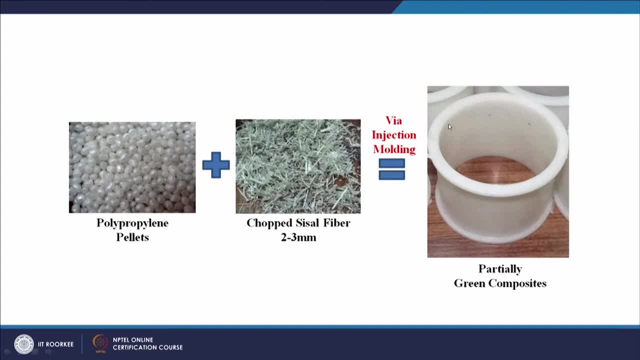 and this is a partially green composite. this will be exact. we can say product: that is the material that we want to make, which is a partially green composite, because polypropylene is a non biodegradable polymer, but the fiber that we are using is a natural fiber. so when 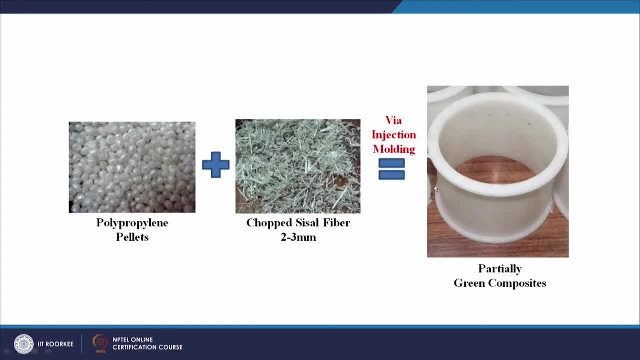 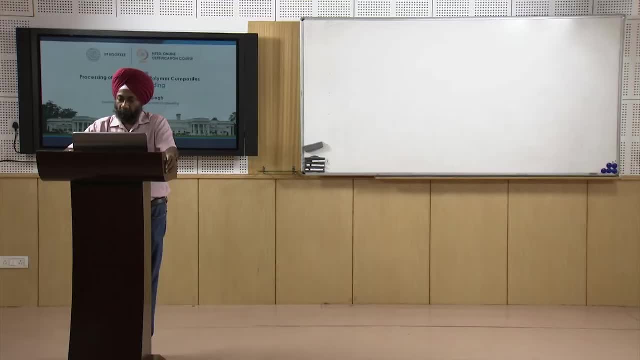 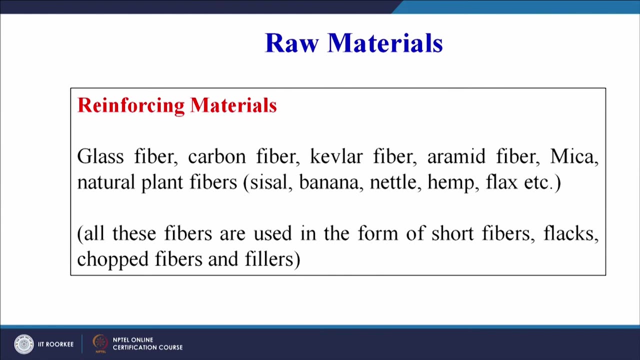 we combine these two in the hopper, we can get a final product of this form. this particular product will be made because of the shape of the mold. Now, what are the reinforcement materials? glass fiber, carbon fiber, cavalier fiber, natural plant fibers, like then, all these fibers are used in the form of short fibers, flakes, chopped fibers and 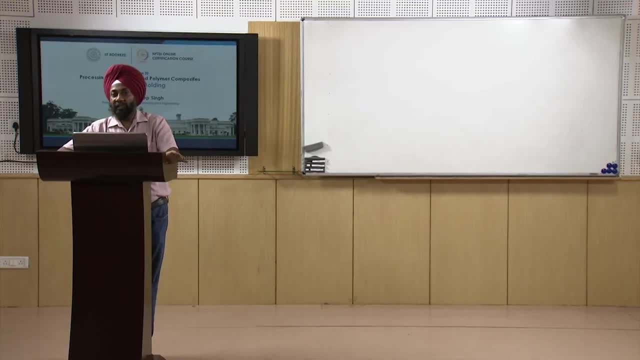 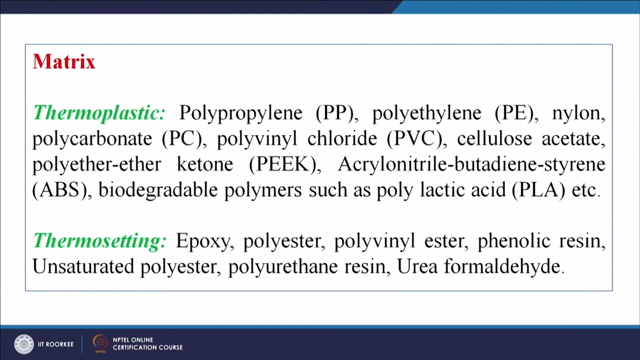 fillers i have already told. injection molding process is well developed for short natural or synthetic fibers. from matrix point of view, thermoplastic and thermosetting resins can be used from thermoplastic polypropylene, polyethylene, polycarbonate, polyvinyl chloride and from 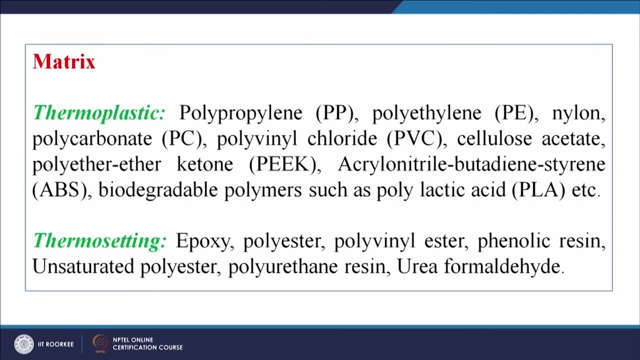 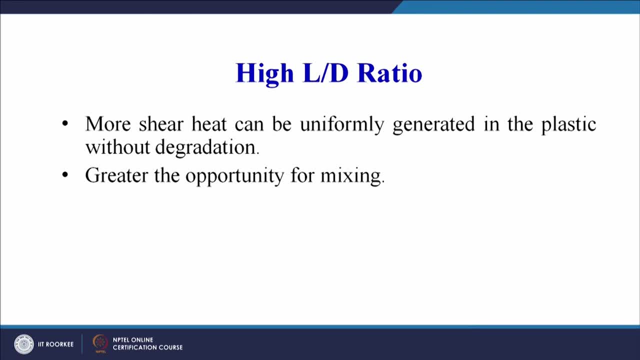 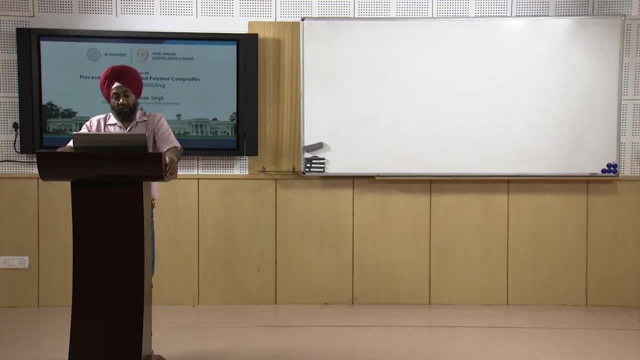 thermosetting epoxy, polyester, polyvinyl ester can be used. now process parameters quickly. let us see high l by d ratio. more shear heat can be uniformly generated in the plastic without degradation and it will. high l by d ratio will lead a greater opportunity for mixing and in order to get the details of these points, i would 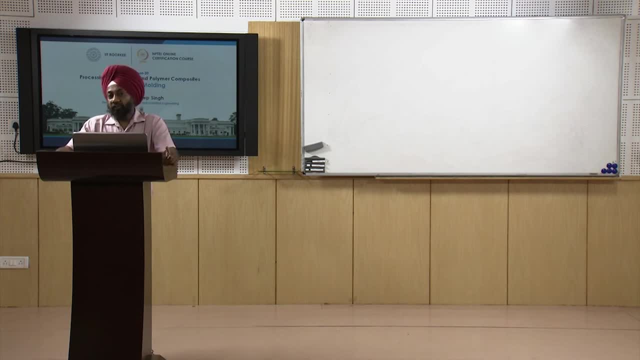 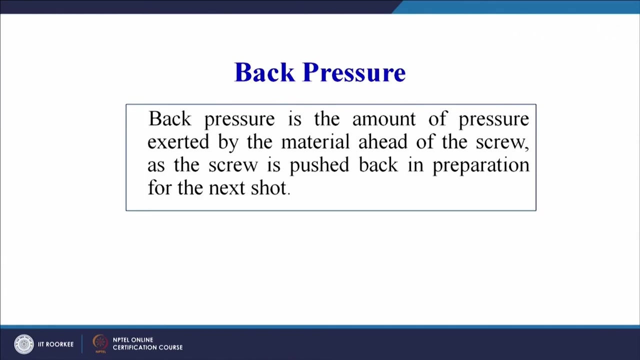 request all of you to refer to our discussion on injection molding. that we have done for injection molding of polymers, because the ah effect of the operating variables is more or less same in case of natural, in case of fiber, reinforced polymers as well as for neat polymers. so back pressure is the amount of pressure exerted by the material, ah head. 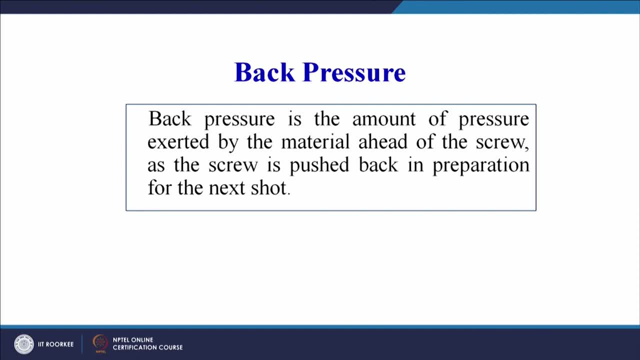 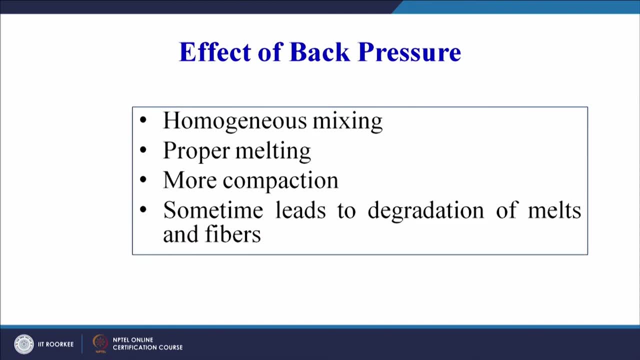 of the screw as the screw is pushed back in preparation for the next shot or the next cycle. then what is effect of back pressure? it will lead to homogeneous mixing, proper melting of the raw material, that is, the polymer, more compaction and sometimes will lead to degradation of the melts and the fiber. so we have to optimally. 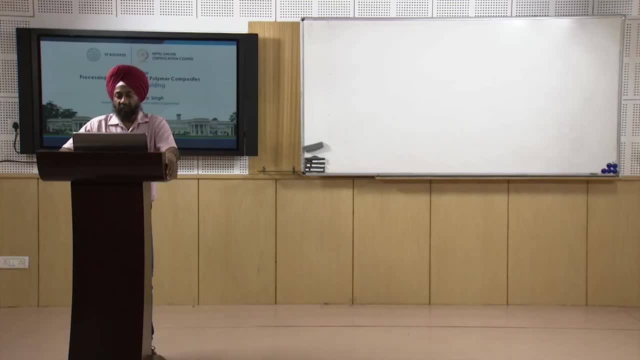 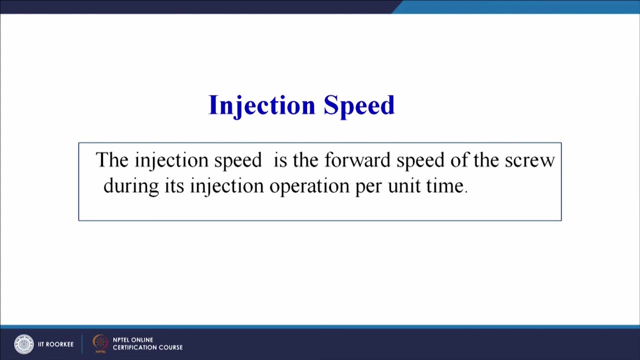 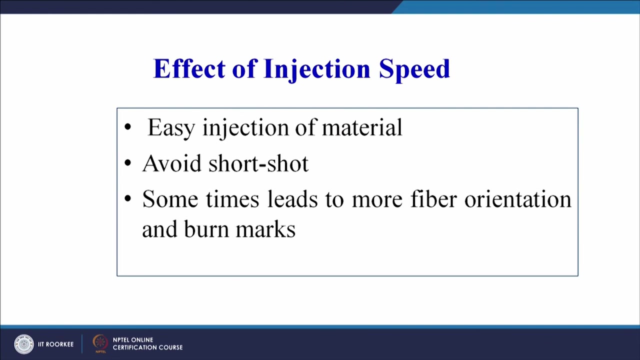 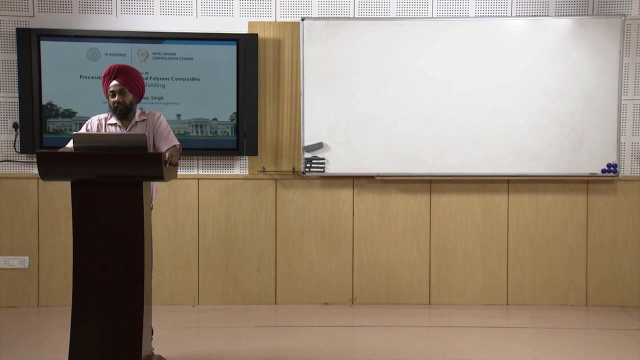 select the back pressure so that no degradation of the fiber takes place. injection speed is the forward speed of the screw during its injection operation per unit time. now what is the effect of the injection speed? easy injection of material. it will avoid the short shot that is ah for ah product may not be formed as per the dimensions, sometimes leads. 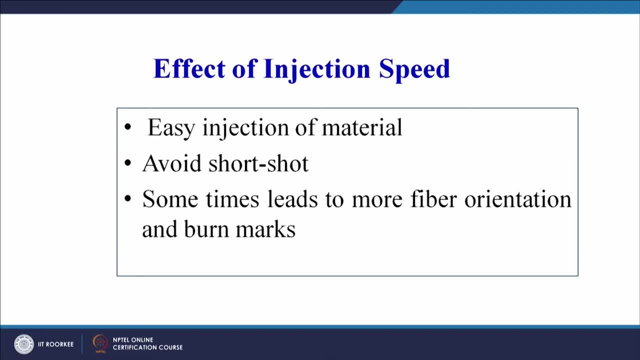 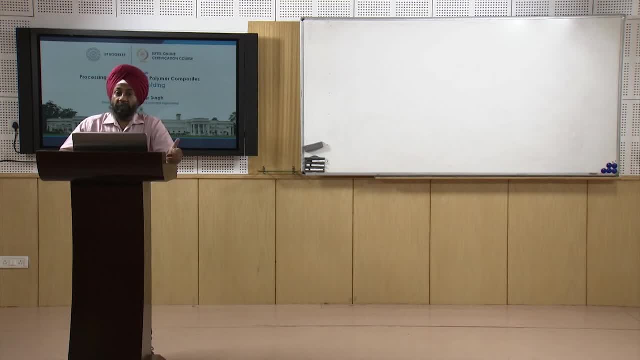 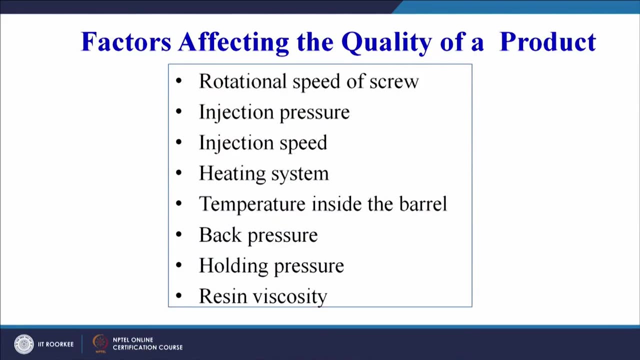 to more fiber orientation and burn marks. so fiber orientation because a high injection speed, we may get a defined fiber orientation so that sometimes may be not desirable in case of a composite products. so these are the factors that affect the quality of the product. very quickly we can read these. rotation speed of the screw injection.